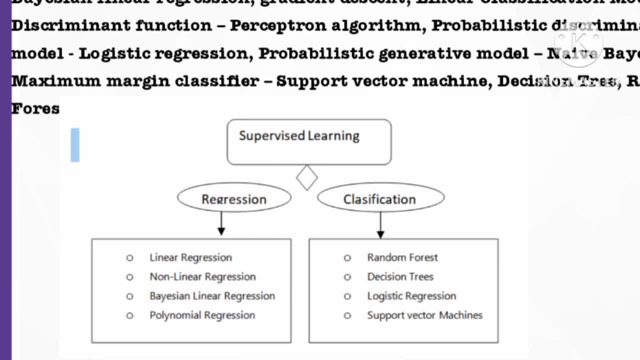 We can easily understand this if we study Classification in Apple. So in Regressions we have Linear Regression, Non-Linear Regression, Base Linear Regression, Parallel Regressions, Logistic Regressions, So Classifications and Random Forums, Decision Trees, Logistic Regressions, Super Hector Machines. 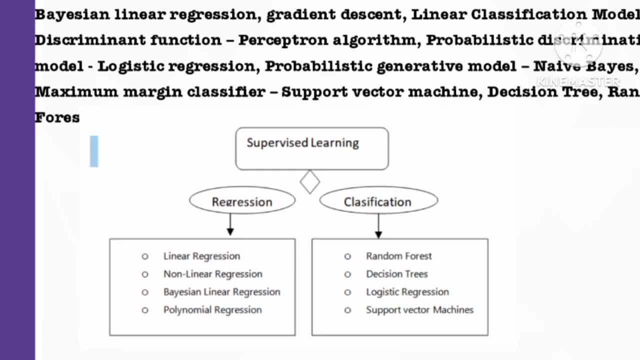 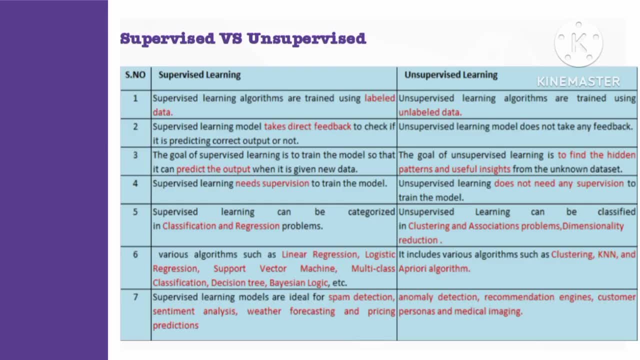 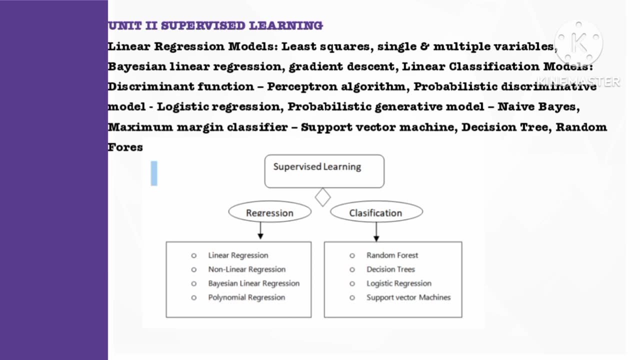 These are the algorithms. We are going to use these algorithms to train a model. So in the 1st one we have seen Linear Regression Models. In this we have seen a method called Least Square. Using this method we have seen what to do in a regression model. 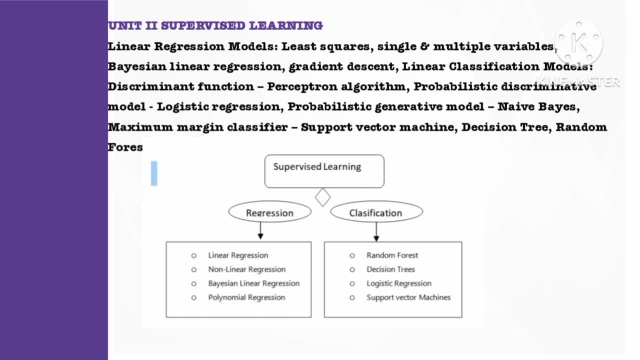 Linear Regression is a continuous input. We have seen a Linear Regression Model to predict an output based on this. For example, If there is a house price, If there are so many rooms, this is the price. If there are 2 or 3 rooms, this is the data set. 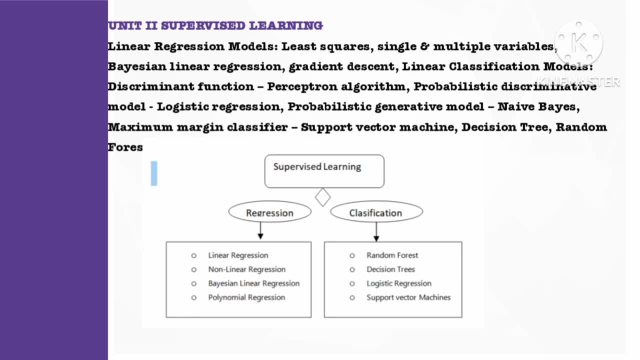 For a building with 10 rooms, we have to predict the price and house pricing. So for this prediction we have to use the Linear Regression Model, the Least Square Method, and use the formula y equals mx plus c to predict the values. 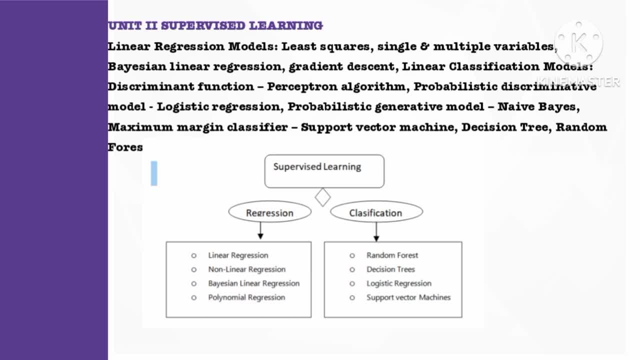 Now we have to find out the values based on the rooms. It is a single variable, So for this prediction we have to use a number of variables, For example for a room, interior and other extra features. This is what we have seen in the Linear Regression Model. 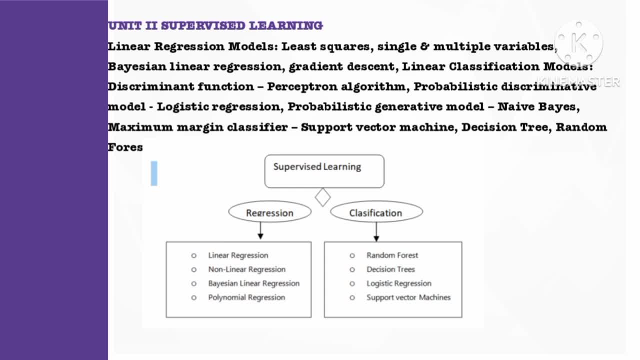 So we have seen Bayesian Linear Regressions. We have already seen how to predict the posterior using the prior knowledge and likelihood. This is what we have seen in Bayesian Linear Regressions. gradient descent: gradient descent is an optimization method in gradient descent method. how do we optimize it? it's loss function. 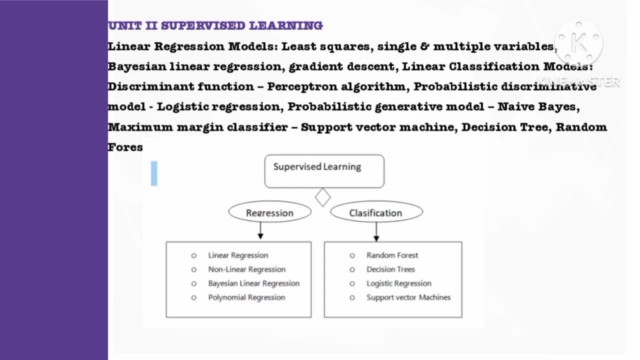 actually, prediction is based on our assumptions and knowledge and the predictions. how is the actual output? the difference between the two deviation is the loss function or cost function. we have to reduce the loss when it comes to the zero. we achieved the perfect model. 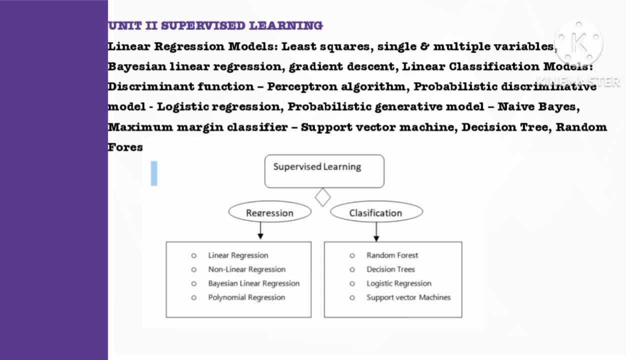 so to achieve the zero we have to minimize the cost function. that's how we optimize in the gradient descent method, which has the least cost function. we minimize the cost function, minimize and optimize the gradient descent to bring the accuracy better. this is what we did before. 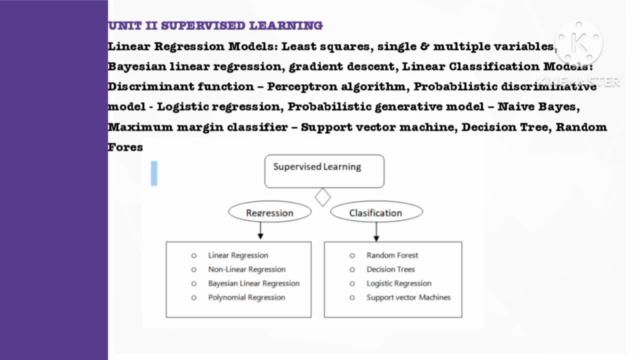 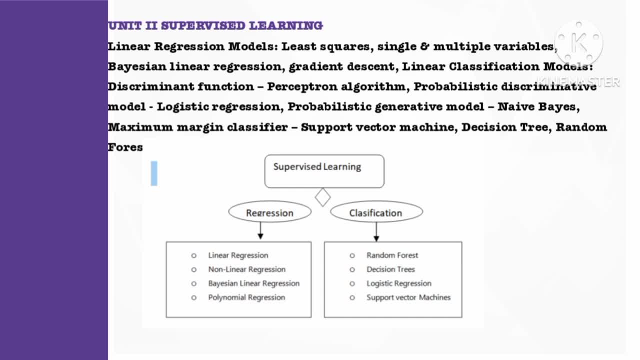 so we have to cover basics and move on to linear classification models. so please listen to these basic concepts. definitely it will help to understand what is this, which algorithm, where to use this particular algorithm. likewise, and also it will help to attend your classes. and also it will help to attend your classes. 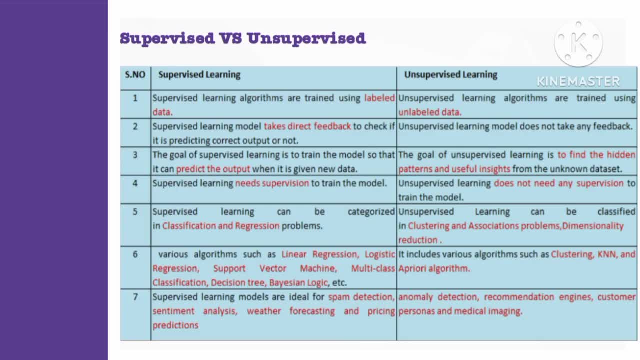 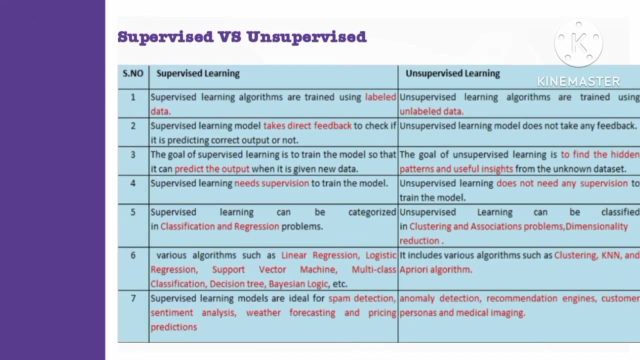 for your examination purpose. okay, so supervised and unsupervised, let's see the difference between these two. it's a kind of method machine learning. it learn from past experience or data produced some output for unseen data or new data. so for that we are using these two methods: supervised machine learning and unsupervised machine learning. 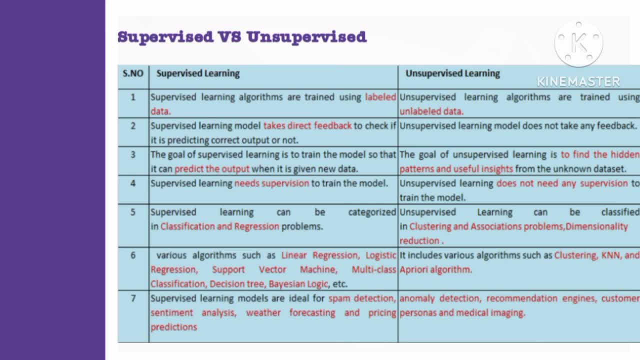 supervised and unsupervised examination purpose. you can use it like that and do the exam so supervised learning algorithms are trained using labelled data. how do we train in supervised learning? labelled data means it's a known data. in unsupervised it trains the model by using. 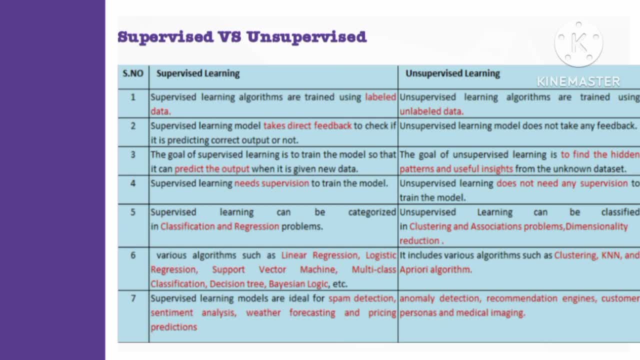 unlabelled data. so in supervised learning it collects feedback. through that it will improve the models or try to use the proper output. unsupervised model doesn't collect any feedback or we can't expect any improvements. the main goal of supervised learning is it should predict the output. 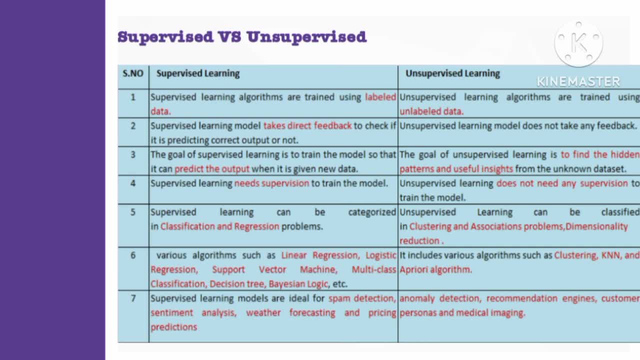 given new data, so we have already trained with some data set. if this is input, then this is output. when we give some new inputs, we have to predict the output. unsupervised learning is not enough just to find out what is the pattern and how it came. 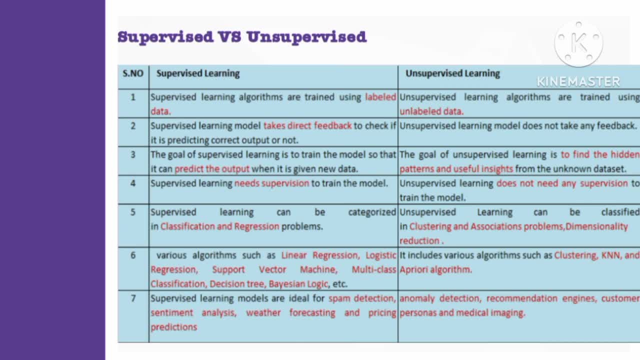 we have to study it in detail. so the goal of unsupervised learning is to find the hidden patterns and useful insights. it should find the insights, so this is where data science will be applied. then supervised learning needs supervision, so that's why it is called supervised learning. 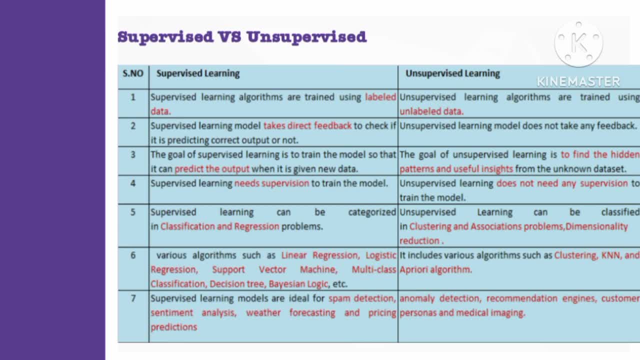 so it needs supervision. based on that, the model is trained. but unsupervised learning doesn't have that. again, we categorize supervised learning as classification and regression. unsupervised learning has classification like clustering, association, dimensionality reductions- all these are in unsupervised learning. 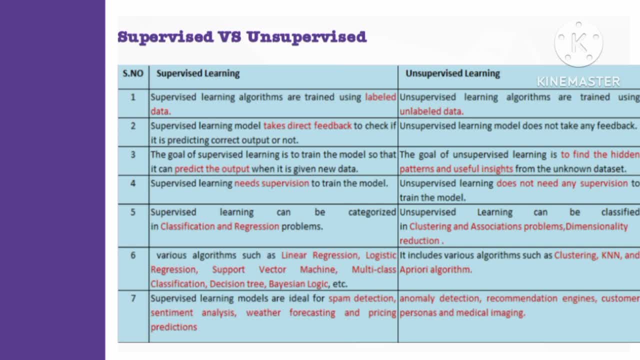 we will see this in detail in the third unit. so various algorithms. what algorithms can be used in supervised learning is linear regression, logistic regression, support vector machines, decision tree, baseline logic. we can use these algorithms in supervised learning, in unsupervised learning. we can use clustering, knn, apriori algorithms. 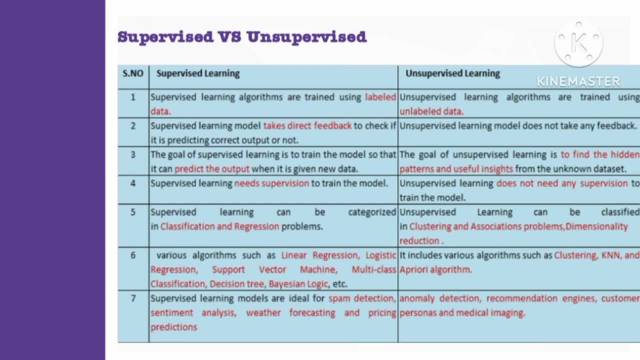 which algorithm to use depends on the inputs and features of the inputs and output, how it should be defined. based on that, we can decide which algorithm to use and according to that, it will give the results. the performance measurements next, supervised learning models. what we use is for spam deductions. 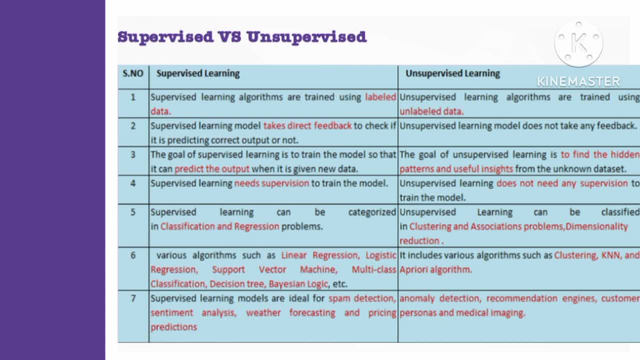 whether it is inbox or spam mail. we use it to identify sentiment analysis, weather forecasting and pricing predictions in sharp market. to get continuous values. we use supervised learning and unsupervised learning, anomaly deductions, recommendations, engines and customer persistence and medical imaging. it is very important to marks and it should. 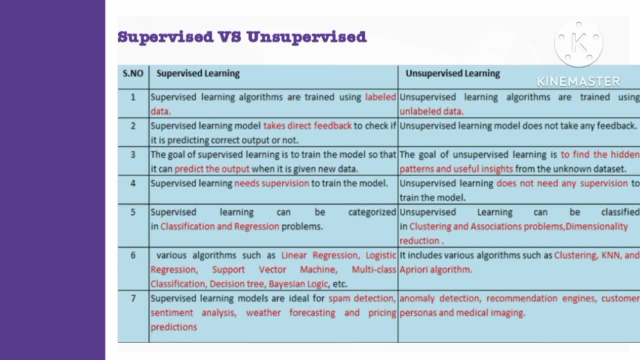 know what is the difference between supervised and unsupervised. so now we are going to see supervised. so it is a label data and it gets the feedback and it predicts the output and it classification by regressions and using these algorithms we have to find the predictions. 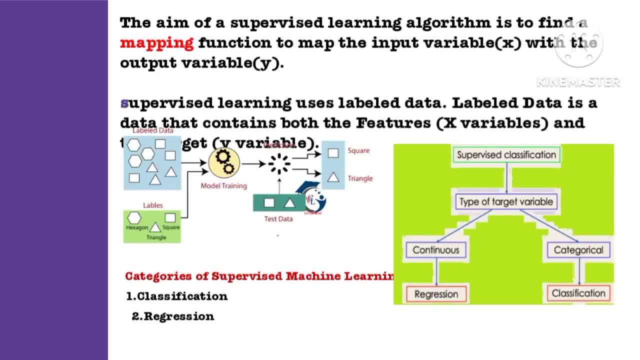 so ok, so the supervised learning algorithm. what it does is it is just mapping the function input variable and output variable. input variable is given as x, output variable is given as y, and supervised learning uses labelled data. so the labelled data has a lot of features of x variable. 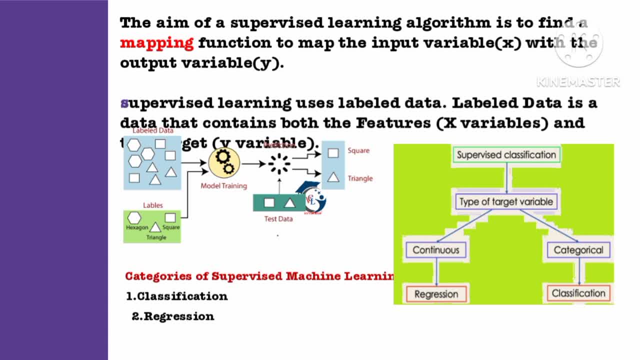 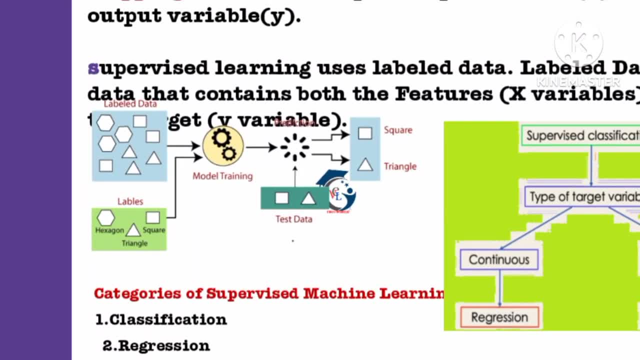 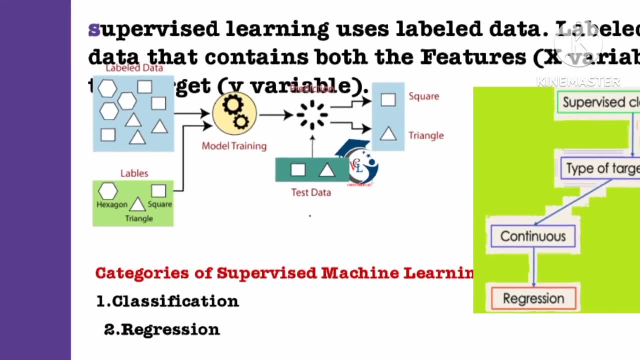 but it has so many features and the target variable or output is y. that is what we have to find out. so the labelled data: we have named the shapes. it is a triangle, it is a square. we have named it as x, we have trained it and given the test data. 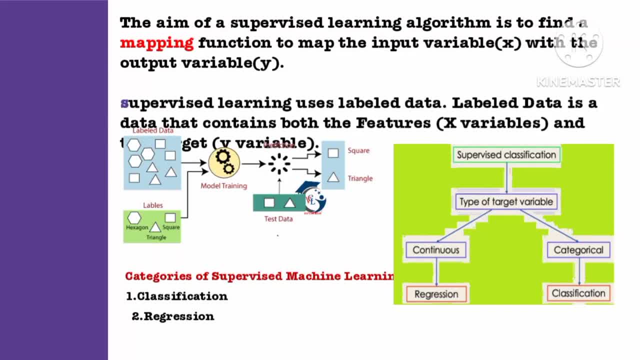 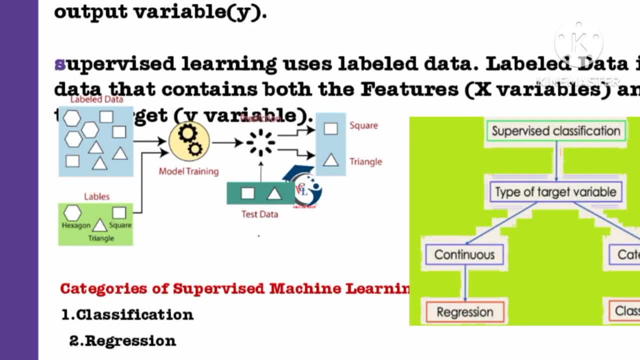 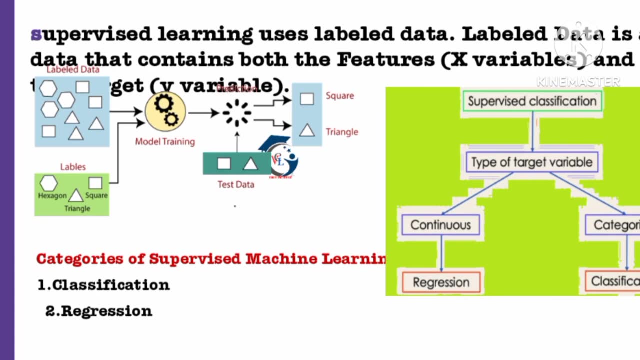 it identifies as square and triangle and supervised learning. is our variable? input variable? sorry, target variable is output. how we are going to find the output? it is continuous or categorical variable. it can be continuous or it can be fixed value, and then it may be the numerical value or it is a categorical value. 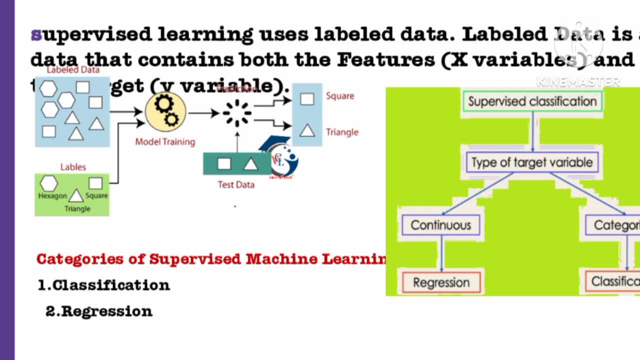 it is based on this numerical value. continuous value: we use regressions. categorical value is classification. what is numerical and what is categorical? we have seen this clearly in data science DEV subjects. what types of data are there? what is the meaning of this? if you want to go through this again, 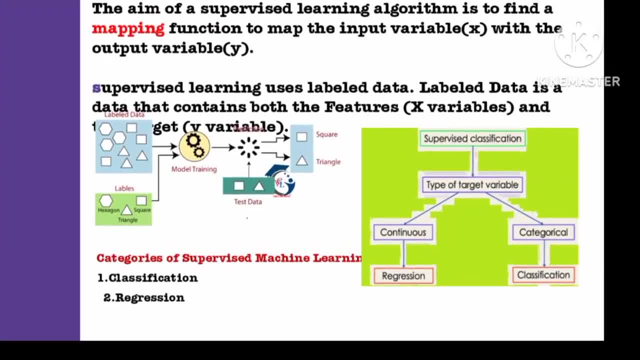 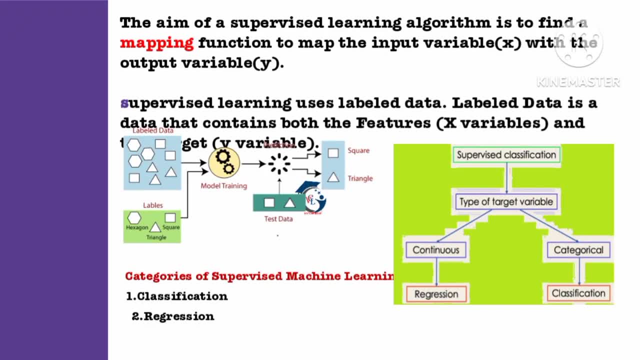 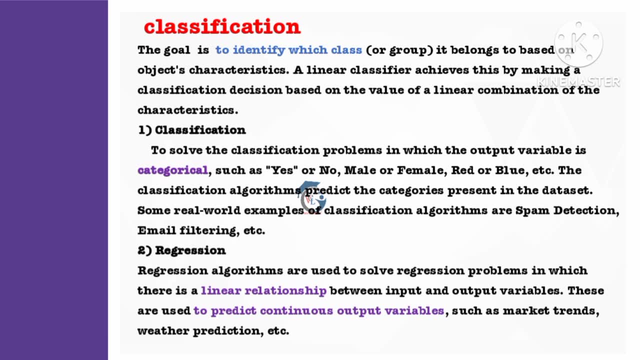 you have to understand and learn. so the categories of supervised machine learning are classification and regressions. we have seen the regressions, now we have to see the classification. so classification, classification: the goal is what class we have to identify, how to identify based on the features or characteristics. 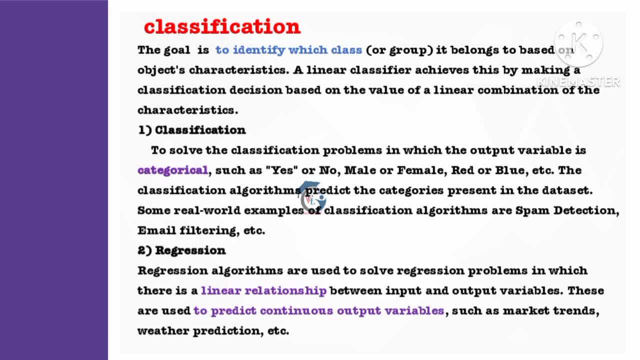 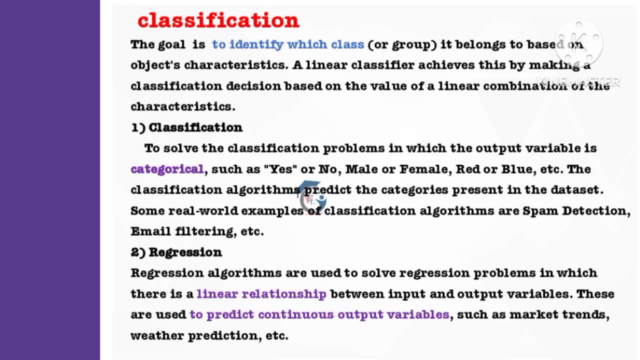 of that object, linear classifier, linear combinations of characteristics. we are going to find out based on that. so classifications is mainly. we are solving a problem. we are using classifications for a categorical value. so what is the meaning of categorical? true or false, male or female, Indian or Japanese? 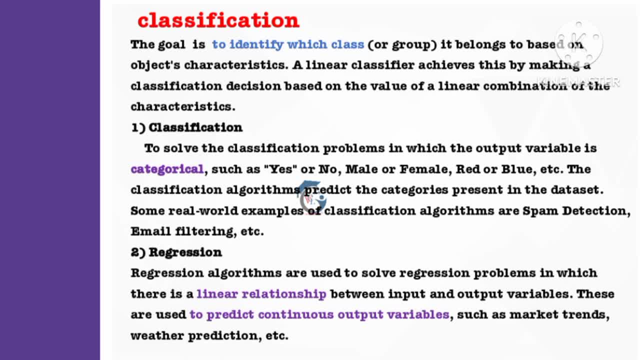 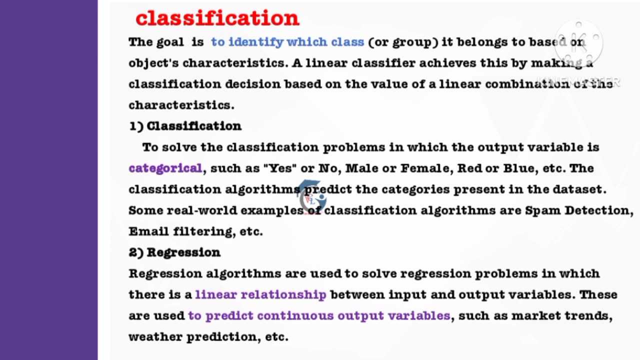 Chinese categories. it may be two or more than two, or more than two. two variables are the categories. ok, next we have regression. what is the use of regression algorithm? it is find the relationship between the variables input variable and output variable. we will find out the relationship. it should be the linear one. 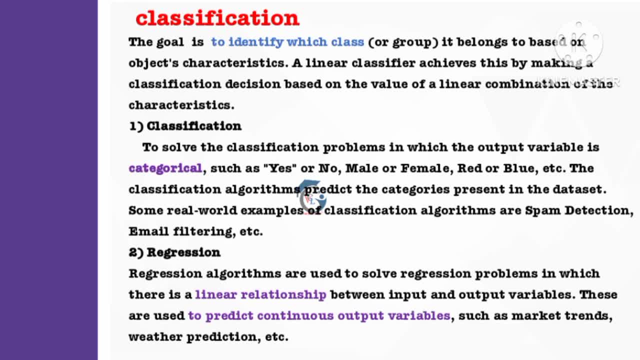 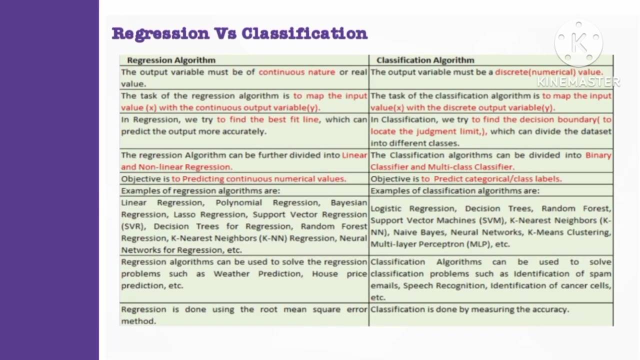 ok, so we are identifying the linear relationship. this is used to predict output variables, regressions um categorical value, classifications. okay, so regression versus classifications. so in the comparisons it's also a important tumor, so regressions for continuous values, and it map the input to the output variable and it's to find the best fit line. 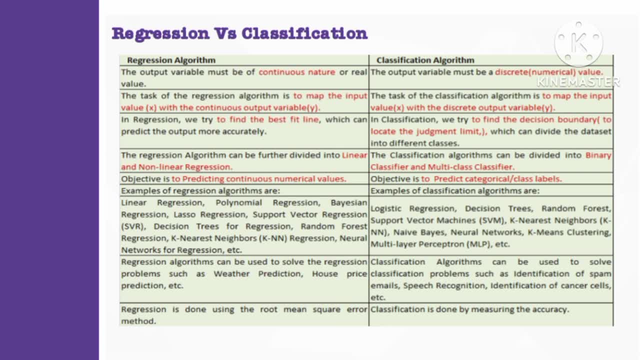 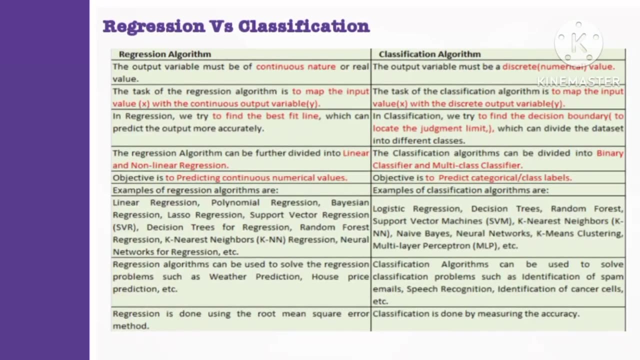 regression, regression or classification is classified into the linear and linear. you know the problem. so the predictions order, sorry, regressions in a pattern or predicting the values, continuous values, 3 predictions, it again. and algorithm is Ponderona, basel, non-regressions, polynomial regression, linear regression and decision tree for regressions, k, n, n for. 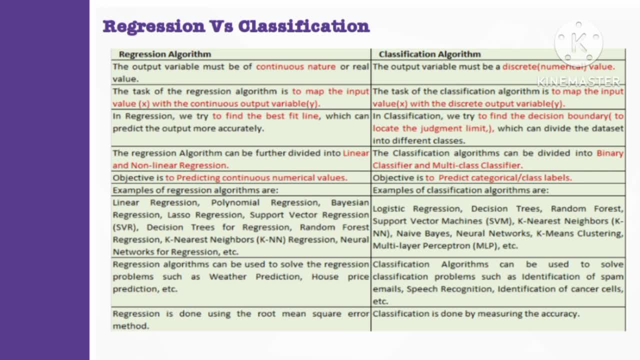 regressions in biri algorithm selection k 4 policies. we are going to classifying these methods, very classifying these activities in lineento in order to judge the optimal data for weather prediction and house price prediction. we use regressions. to improve regressions, we use root mean square error method. 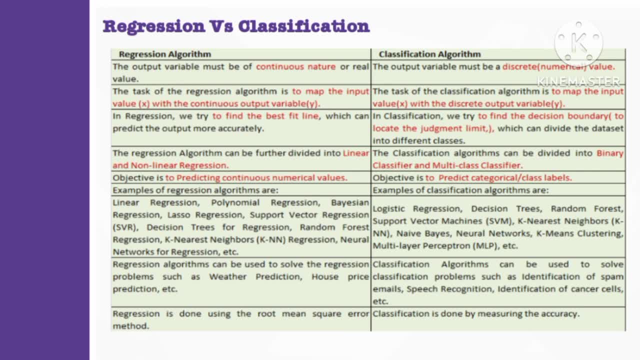 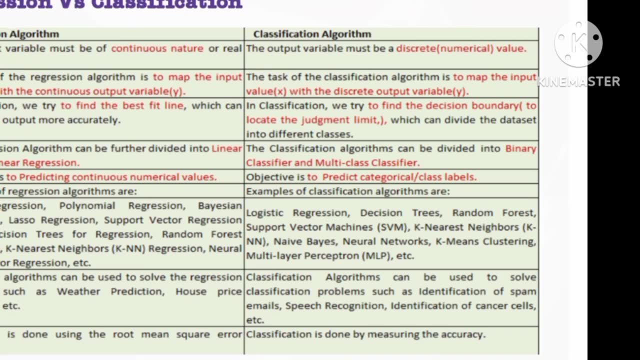 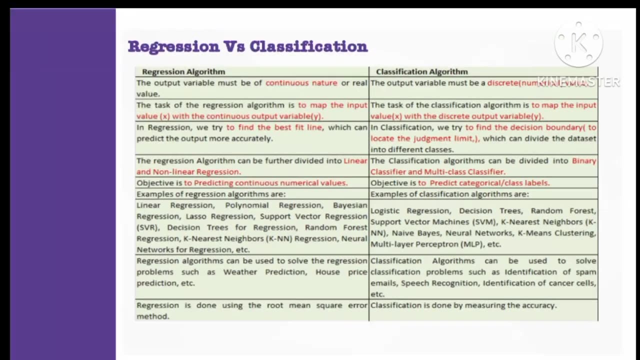 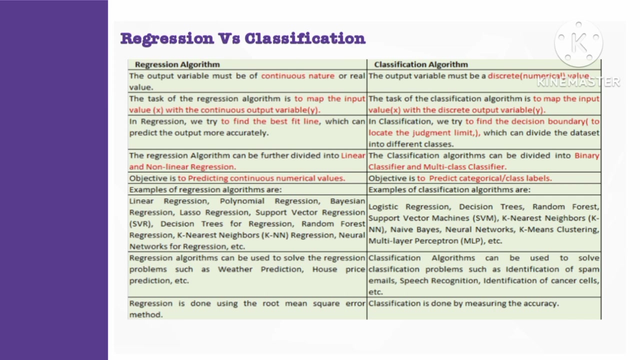 to optimize it. output variable is discrete or numerical and task is mapping x and y values. in classifications we use decision boundary. this is the major one in classification algorithm. we use binary classifier and multiclass. objective is to label which class to label. we use decision tree algorithms, logistic regressions, knn. 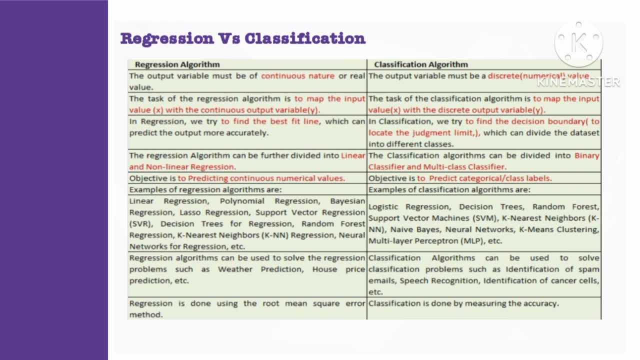 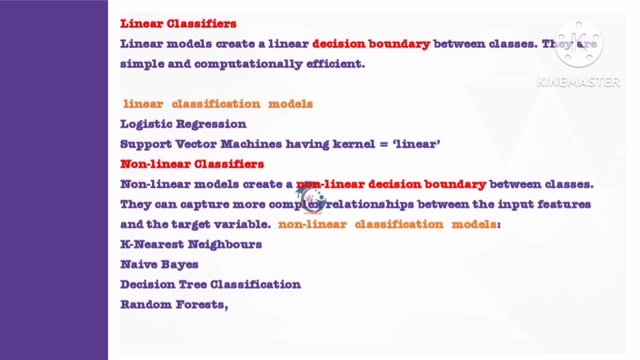 name base. k means clustering. we use this for identifications like spammer mail, speech recognition. we use this for classifications to improve accuracy. ok, shall we move to the next? now we will see classification in total. what is classification? classification is to identify which class has many inputs. 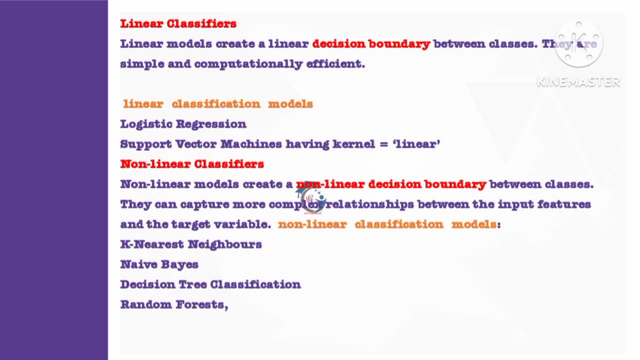 for example, if we have citizenship, we can use some basic to find out if they are indian, chinese or japanese, for example. if they are indian, the person's colour will be like this. person's hair will be like this person's characteristics will be like this. or indian people's nature will be like this. 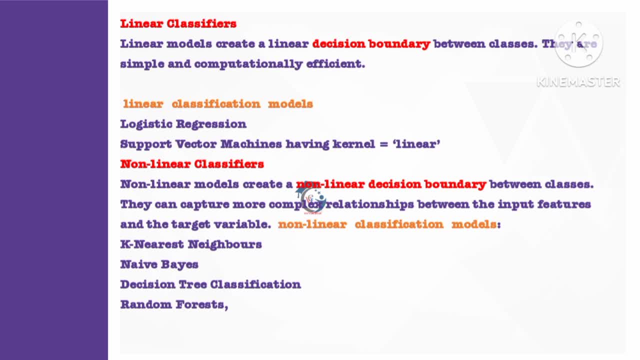 their food habits will be like this. so, likewise, based on some features, we can identify whether the person is indian or chinese or japanese. chinese will be like this. japanese will be like this. so, based on physical characteristics or some food habits, we can identify like this. so like this. 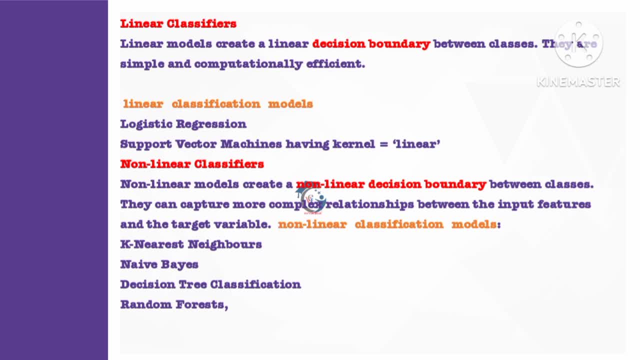 we can identify in which class they will come. we can identify in which category they will come. this is the main theme of classification. ok, so again, earth is categorized into two: linear and non-linear. we can see what is that. so, linear models: we have to create a decision boundary. 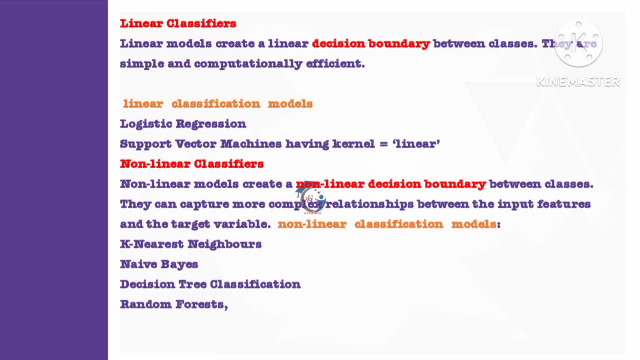 if it is within this boundary it will come in this class. if it crosses this boundary it will go to another class. we have to identify that. that is linear classification, so that decision boundary line should be the linear one. linear means we know there should be a line. 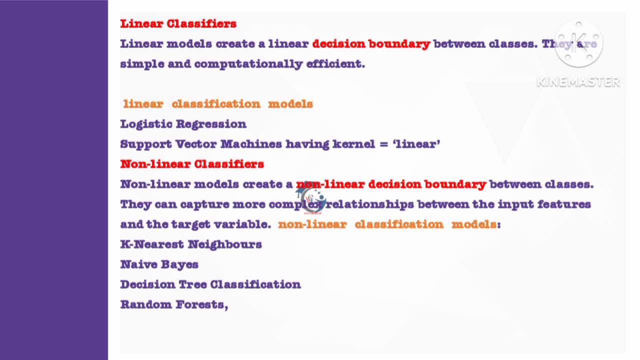 like a straight line. ok then linear classification models. whatever we can use logistic regressions and SVM. we can use linear classification, non-linear classifications, non-linear decision boundaries. we have to see how it will be. in linear classification, the decision boundary will be a line, as Vadivelu says. 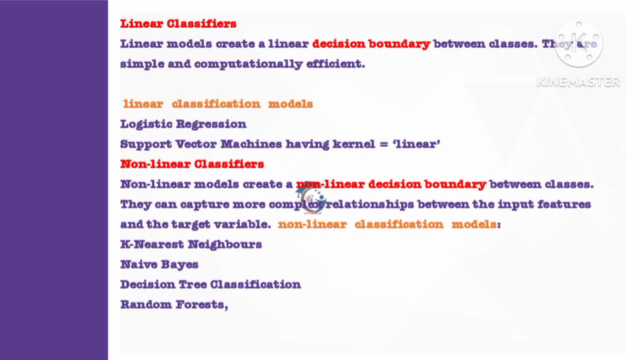 you should not cross this boundary. I will not cross it like that. we can fix a line and the variables inside that line are categories and the ones out of the line are categories. like this we can find out. this is linear classification, non-linear is not like that. 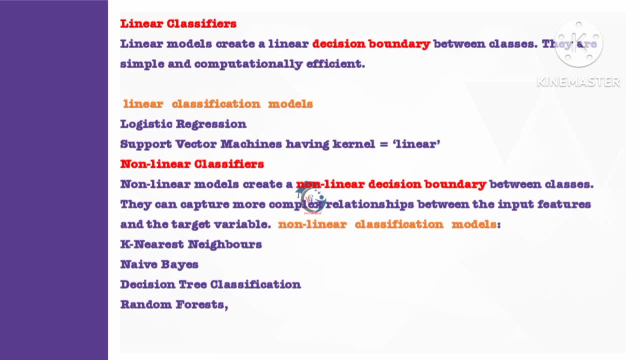 everything is mixed, we can't fix it with a straight line, like a group, like a circle. you would have studied Venn diagrams A, B, C, like that. so wherever it is, we can circle it and make it a category like that. likewise it will be non-linear. 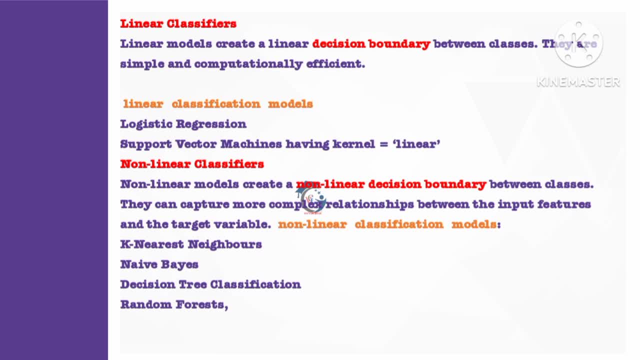 ok, it will not be a non-linear straight line. it may be the curved line or circle or ellipse, any curved based boundaries. ok for this. the models we can use: KNN, Naive based decision, tree classification, random forestry. we can use these for non-linear. now, what have they given us? 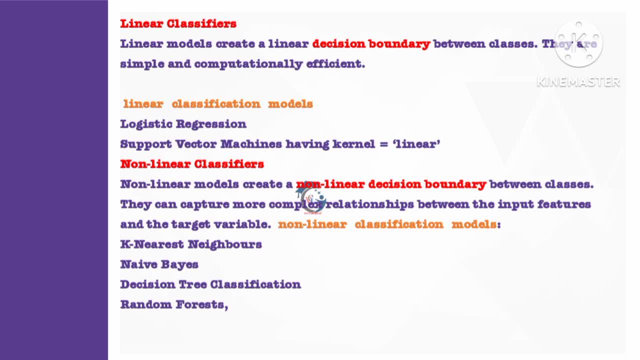 linear classification models. linear classification models. so now I think you are clear what is classification, what is regressions, what is supervised learning and what are the algorithms between linear and non-linear? which algorithms can be used linear? what is non-linear? what is classification? you will be clear. 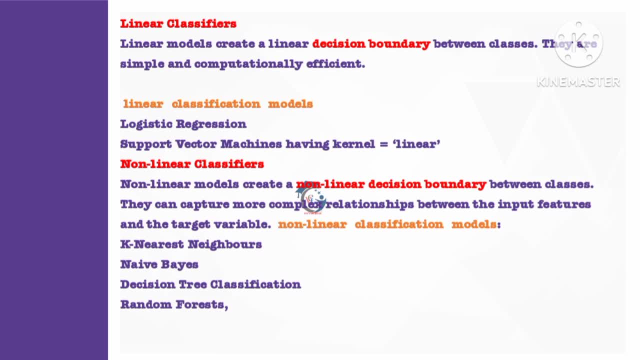 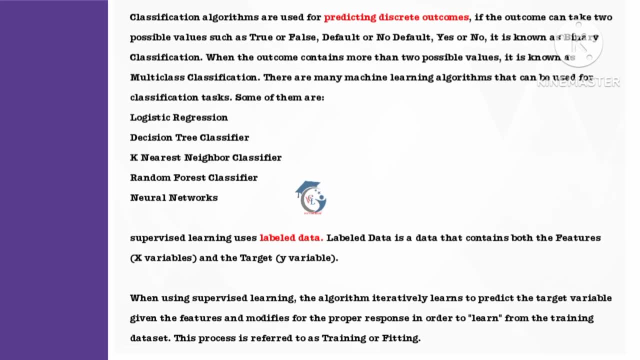 ok, now we will see in detail. ok, so classification algorithms are used for predicting discrete outcomes. ok, so you can read some theory for examination purpose. I just try to provide some content. that is why I have given all these main keywords are given in colour you can use. 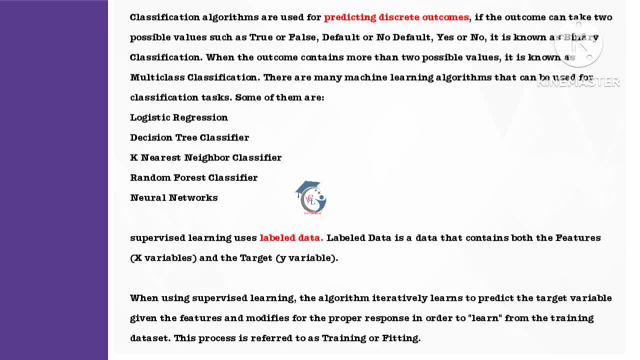 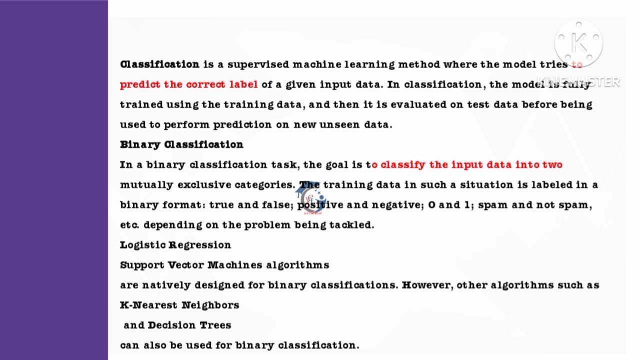 these and do your examinations better. ok, for understanding purpose, you know what is classification and supervised. what is? its input features and target variable is y variable. these are the algorithms. ok, so classification is a supervised machine learning and it is for predicting the correct label. what category is it? 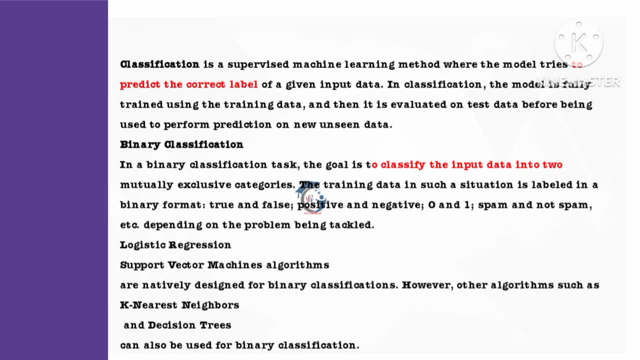 categories. to find out is the main theme. so now, as we said, in classifications there are some categories. first one is binary classifications. if the category is two means it is binary classifications. that is all ok. it is like true or false, positive or negative, zero, or one spam or not spam. 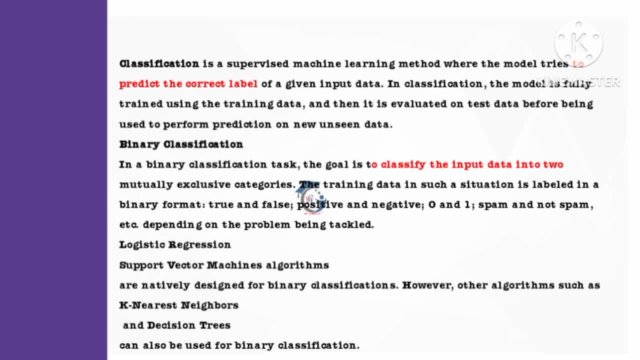 Indian or American or yes or no, like this. if there are only two options, that is, binary classifications. ok, so what algorithms can be used for this? logic, regression, support recognition algorithms, decision trees. we can do these binary classifications. if there are more than two, it is multi class. 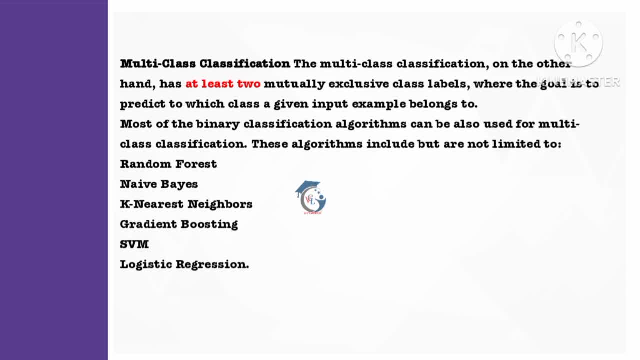 classifications. ok, so American, Japanese, Indian, Chinese, like this: if there are more than two options, it is multi class. again, we can apply binary in multi class because there are two more than two options. so we have two options in this random forest naive base cane and these algorithms. 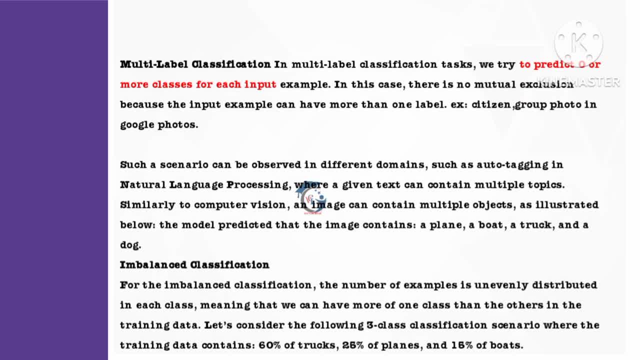 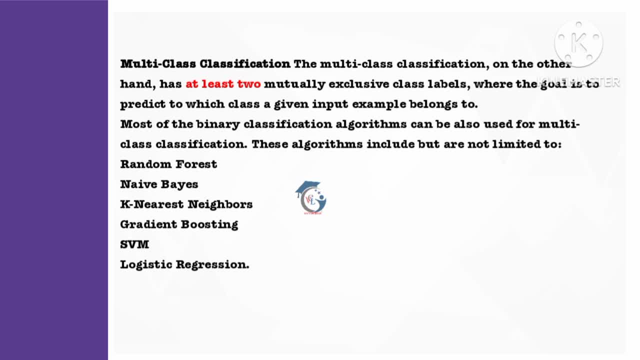 can be used in multi class classifications. then multi label classification, multi class classification: here we see there is multi label classification. there are many differences between these two. now I am giving a human picture, there is only one person. if I check in one picture, there is a group. 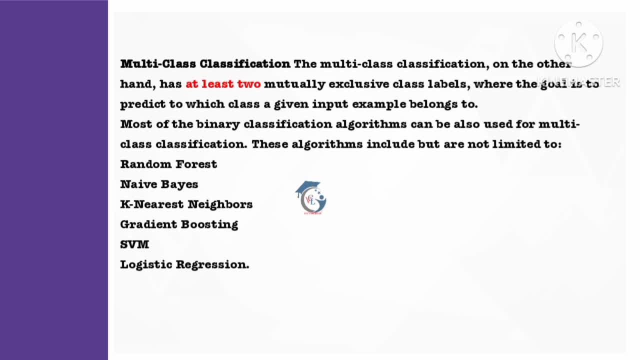 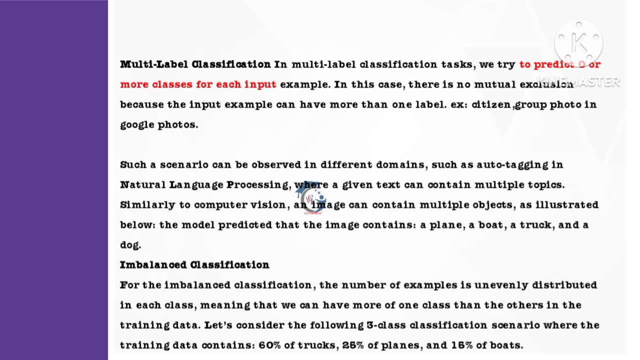 of people that photos, all the people: Indian, American, Chinese, Japanese. how can I do multi class with that photo? because there are four options. that is called multi label classification. ok, so more than one classes for the name. you can name the name. you can name the name of. 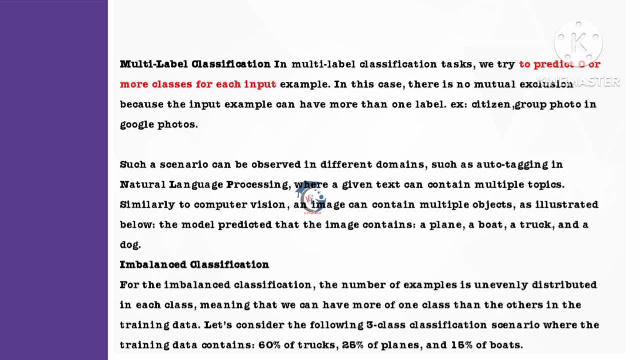 the photo of the photo and the name for the photo. so the name. we have to name the photo. we Now we see in phone previous year where we were the photos we saved. When it comes in the name of the particular person is given and the name related photos are shown. 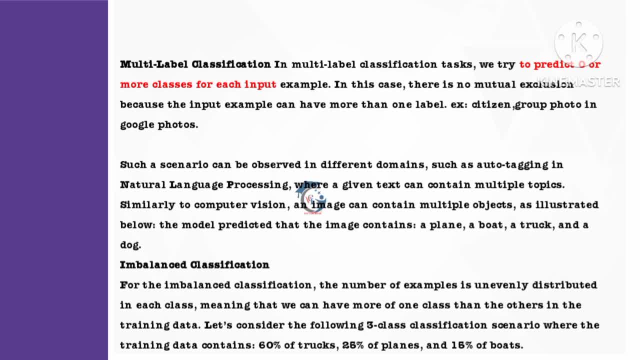 Now how it happens is: in that particular photo, each person has been labelled with a name, So based on that it is generated. That is the best example for multi-label classification. That is one input. it has so many features. each one is in one category. 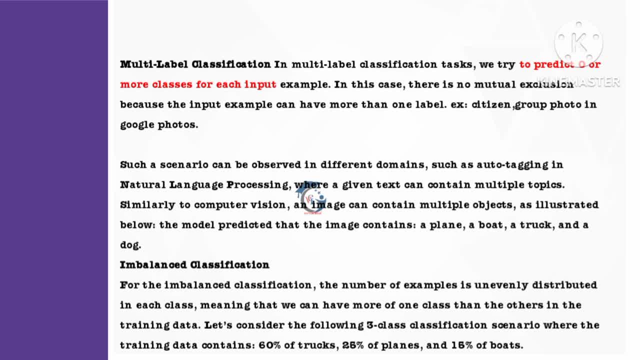 That is what you do for multi-label classifications. Next, imbalanced classifications. This is not evenly distributed. This is not evenly distributed. This is not evenly distributed. For example, an Indian father or a Chinese mother if they have a baby? 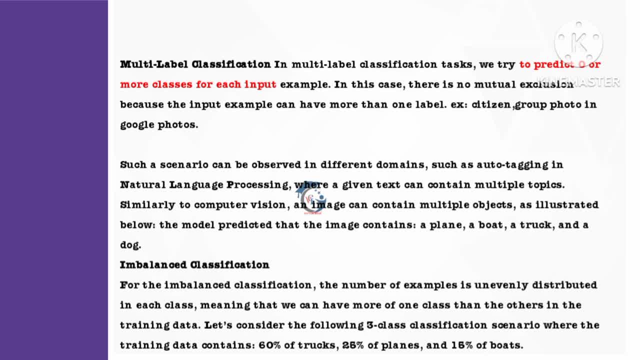 if they are like 50% Indian or 50% Chinese. we cannot analyze them by using only physical characteristics. Even if we say so, we cannot give a perfect result on a percentage basis. That is imbalanced classifications. We cannot do a proper classification. 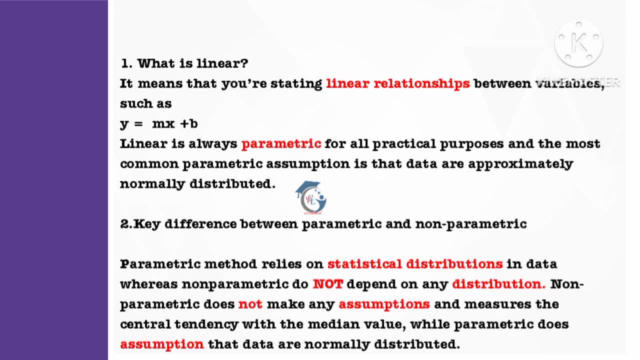 These are the two marks and for clarity I have given this, Why I have given two marks and importance separately and not in between. if you know all these, you will understand this concept. That is why I have given this What is linear. 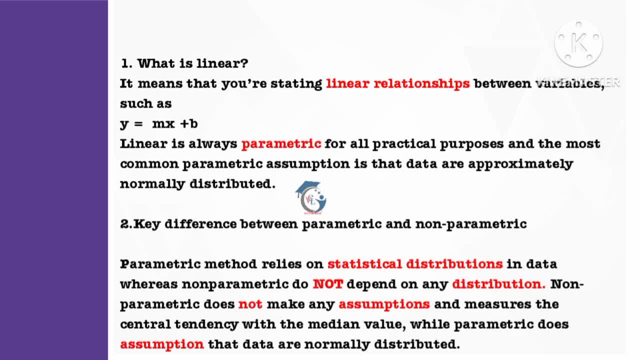 There is an input variable x and an output variable y. If the relationship between these two variables is linear, that is linear. Another name for linear is parametric, That is, we can identify a linear relationship by using a measurable variable of x and y. 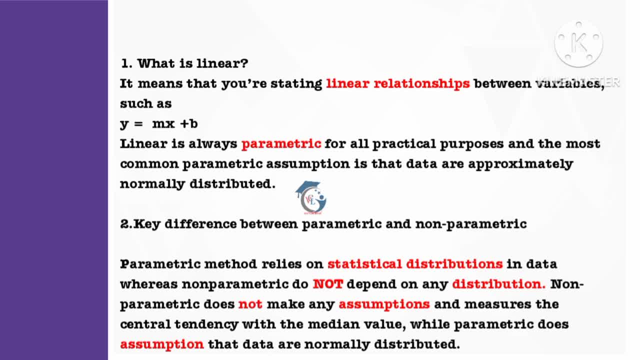 That is linear or parametric. Next, we have asked the difference between linear and non-linear. So parametric is linear, It has a static distribution, But non-linear does not have a proper distribution. In linear we cannot bring any assumptions. 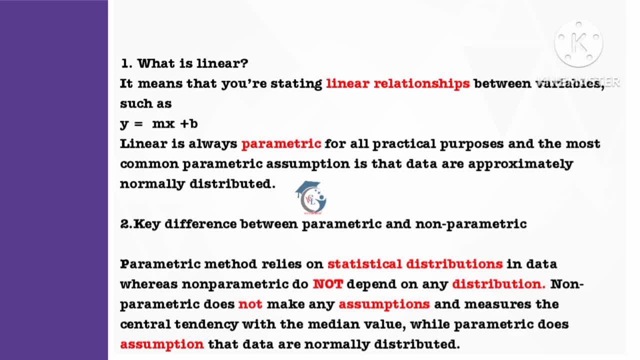 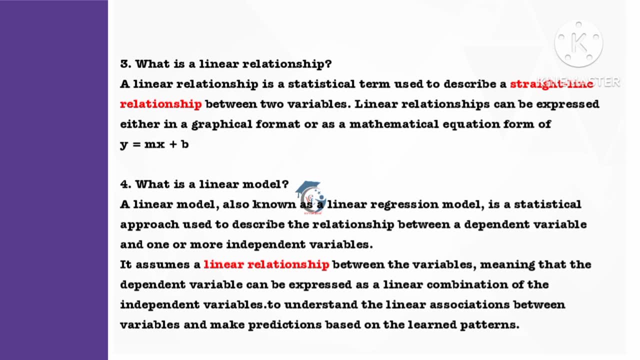 But in non-linear we cannot bring any assumptions. But in non-linear we cannot bring any assumptions And it measures the median value. So this is the difference between linear and non-linear. Linear relationship is when we draw the relationship between the input and output variables. 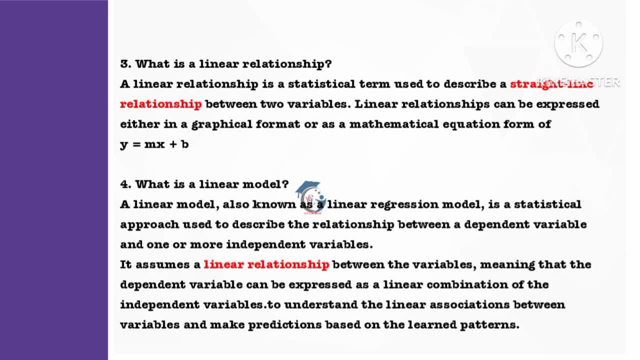 and the line is a straight line, that is a linear relationship. So that is what we did with the formula y equal to mx plus b, And linear model is the linear relationship between the input and output variables, And linear model is the linear relationship between the input and output variables. 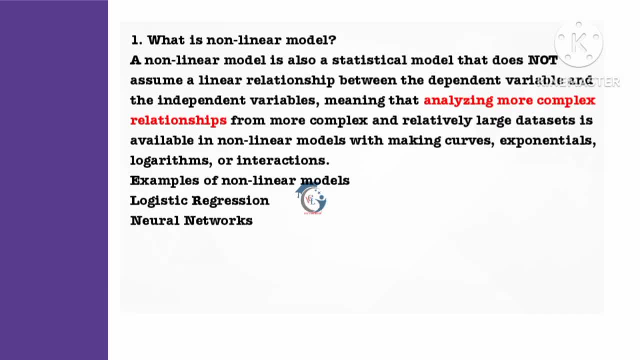 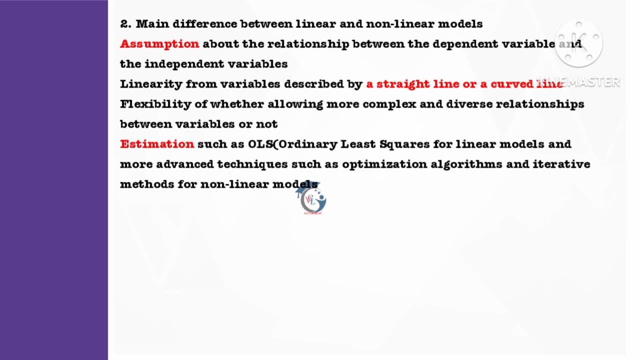 Next non-linear model is: when we cannot find the straight line, the best fit line or the curved line, Then we can draw the non-linear model. So the difference between linear and non-linear, Again, linear is the straight line. 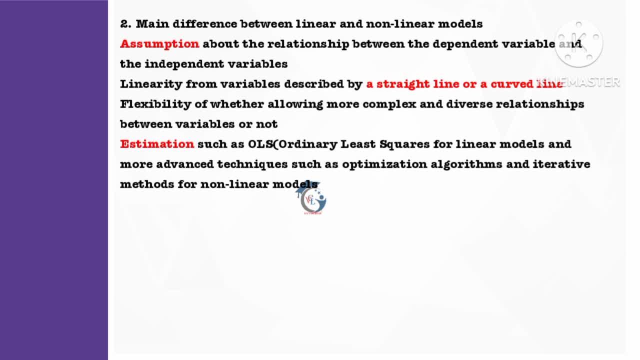 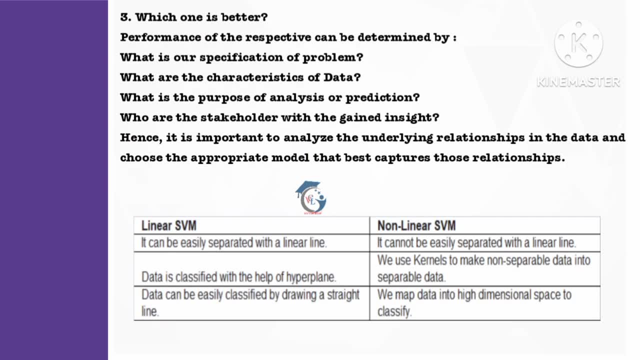 Non-linear is the curved line And non-linear is the curved line, So we can identify this by using least-square methods And, which is better, we cannot say So. the specifications of the problem, the features of the input data and what is the purpose. 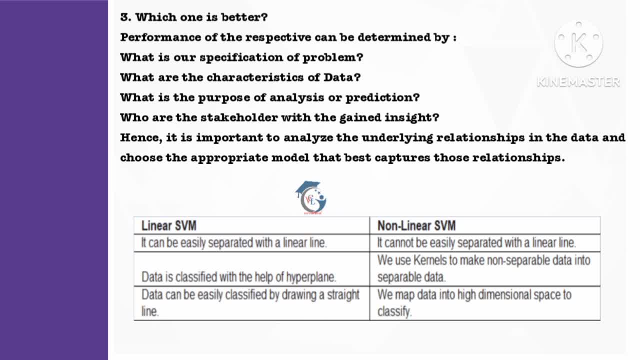 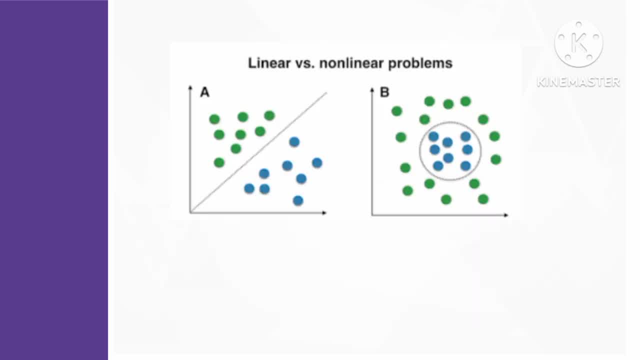 we can analyze and bring them in predictions. Whatever we can base itself on, we can tell whether it is linear or non-linear, or which one is the best. Okay, And yes, This is to explain you the difference between linear and non-linear. 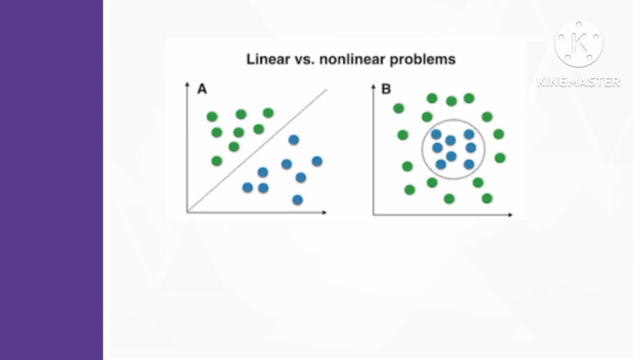 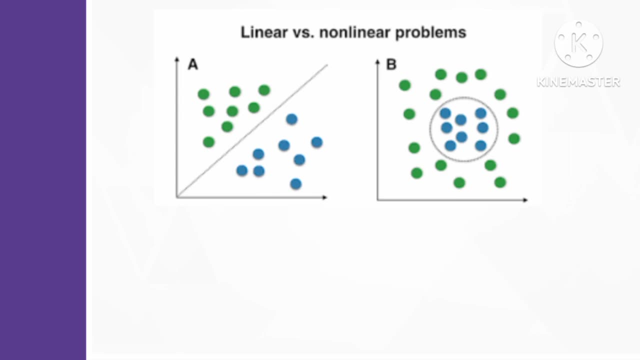 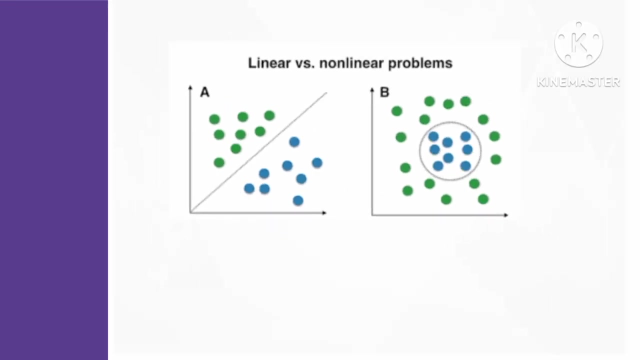 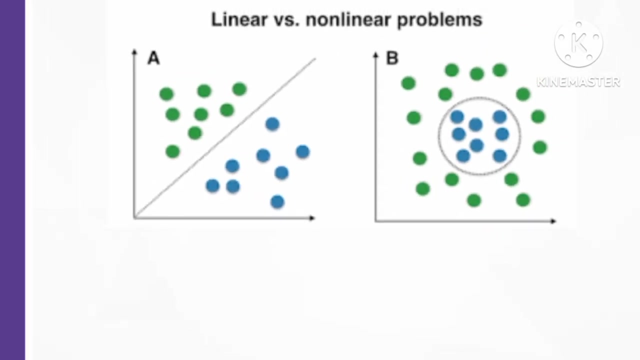 Green and blue are categories. This line can be divided into two lines, So we can differentiate between green and blue by using this line. But in this diagram green and blue can't be differentiated by using a line, So we have to use a circle for this. 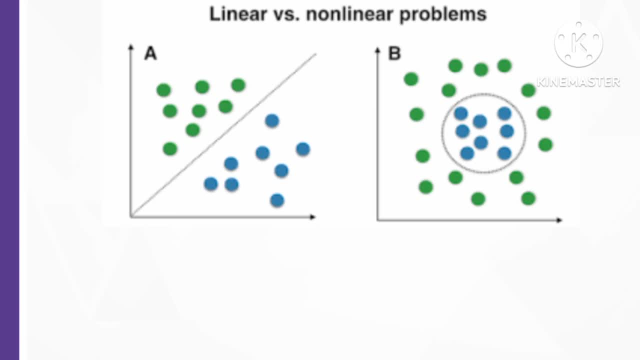 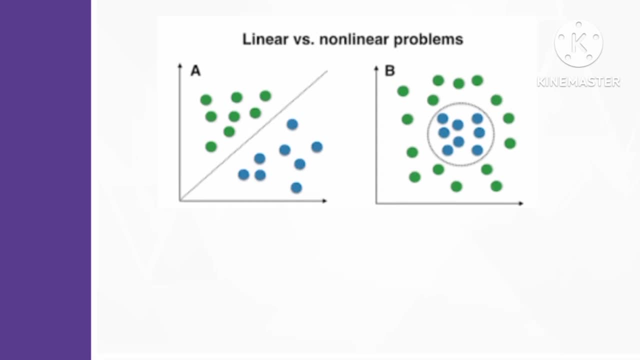 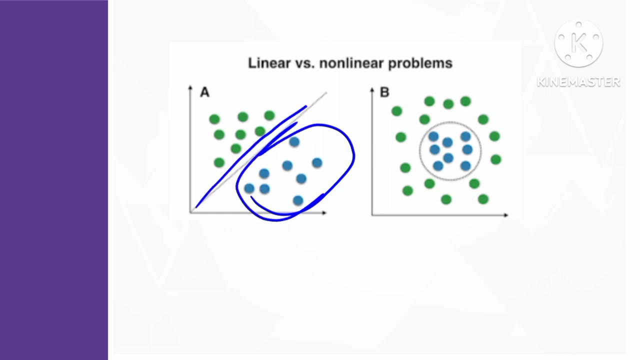 Blue is the interior and blue is the exterior. So we have to differentiate between these two lines. A is linear and B is non-linear, So we can differentiate between these two lines by using a line. So we can differentiate between these two lines by using a line. 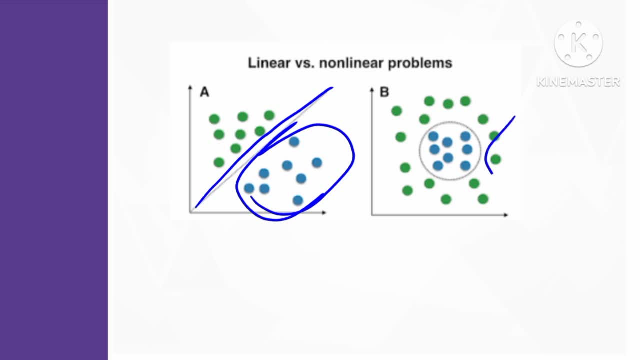 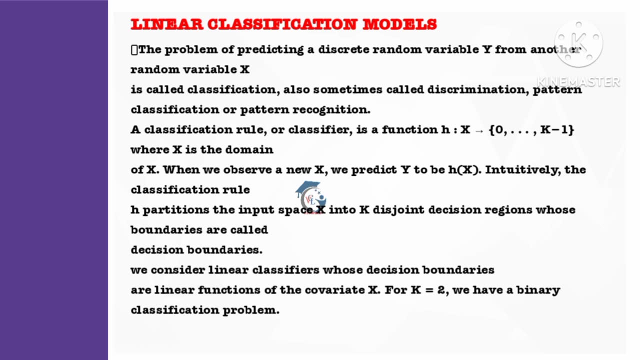 This is non-linear. This is non-linear. ok, so next, linear classifications model. now only we will come to the title. actually, today's topic is linear classification model. ok, but previously, if you don't know this, you will not understand this. ok, so x is the input variable, y is the output variable. 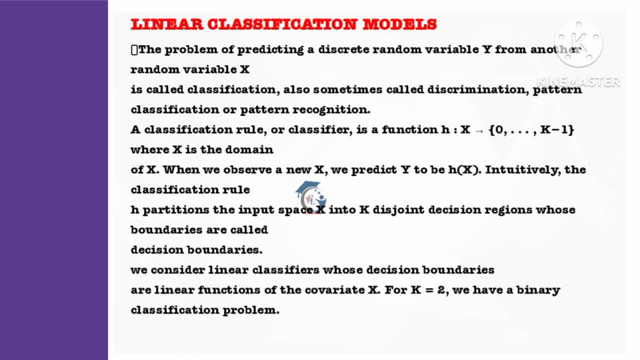 based on some features. we classify classification. classification- another name is discrimination- and pattern classification or pattern recognition. all these will have the same meaning. x is the domain and particular variable is the input feature. y is the prediction. we follow some rules for classifications, ok and decision boundaries. this is the main thing in classifications. 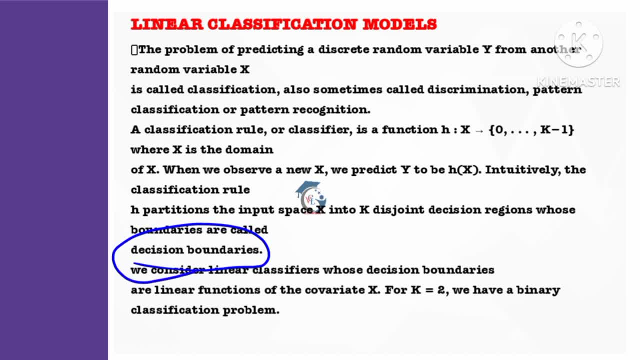 any line or circle that is based on decision boundaries. k is equal to 2 for binary classifications because k is the number of classes, how many groups are there, how many categories are there? that is what we call k. binary has 2 categories. these are some important notations. 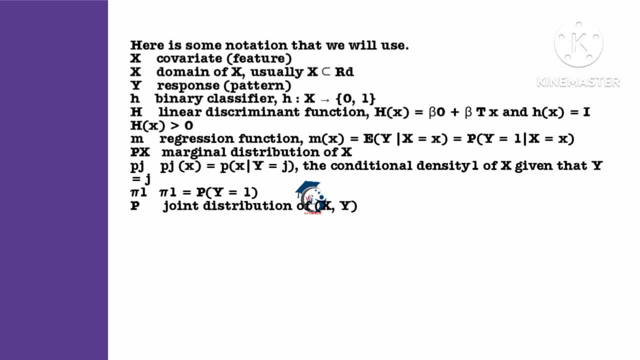 mostly used. x is covariance formula is equal to mx plus b. one variable of x is x, more than one variable is m1, x1, m2, x2. these are the coefficients. we have to find out. next, y is a response or pattern. we have to find out that. 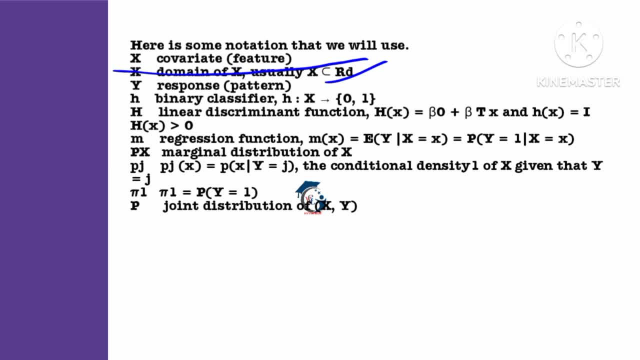 we have to find out the pattern. next is binary classification: 0 or 1- there are two options- and linear discriminant function. we will see this. next is regressions. we have already seen this. we will find out m. in regressions, y is equal to mx plus b. 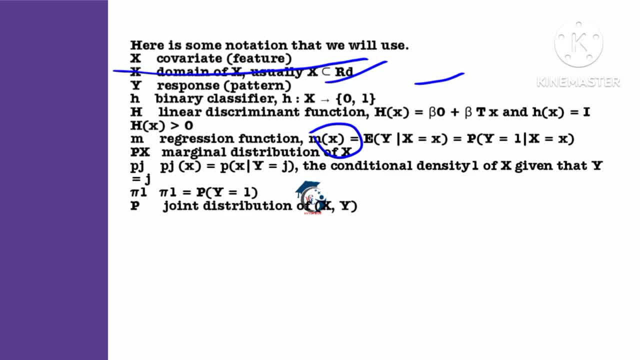 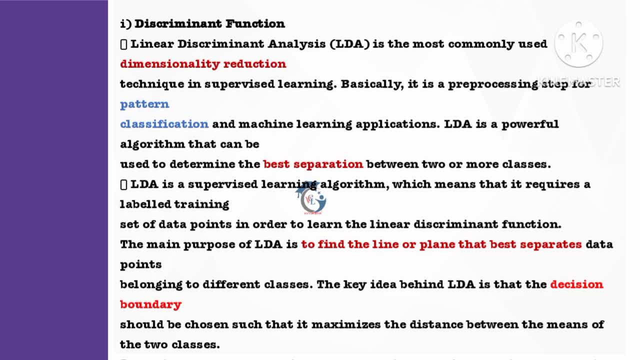 we will find out. m next is. next is discriminant function. in discriminant function, we have linear discriminant analysis. linear discriminant analysis mostly used for dimensionality reduction. we have already seen this in DEV, when we analyse a data when there are more than one field. 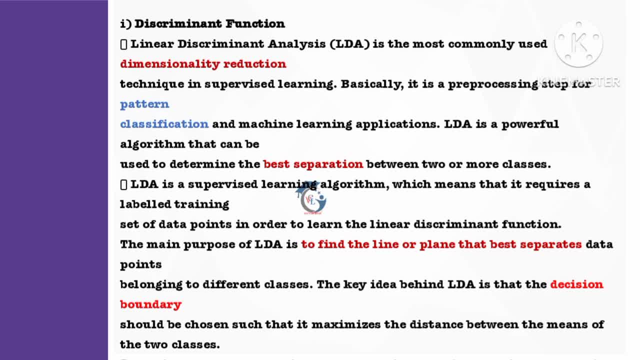 or columns, we cannot get a conclusion. so for a particular decision making we can work with some of the fields. so we have to do dimensionality reduction with this data. so for that purpose we can use linear discriminant analysis and make it easy. ok, so to classify the pattern. 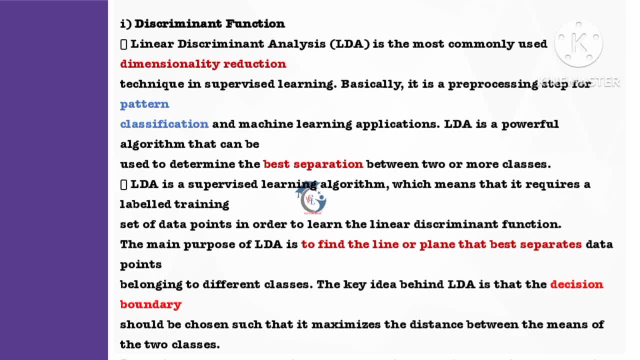 we have to use this. ok, so in this, what we have to do is best separation. ok, so we have to use something to do the separation. this is this class. this is this class. on what basis we have to do the separation, that is, to determine that we have to use this discriminant function. 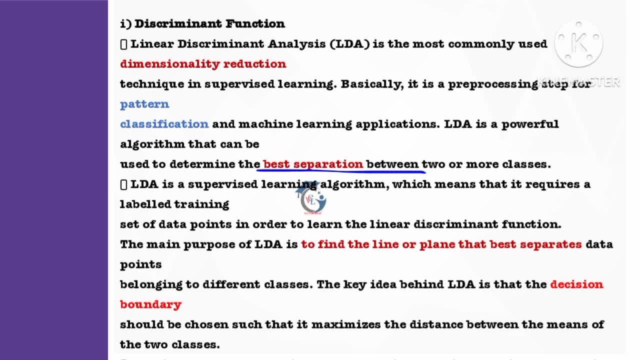 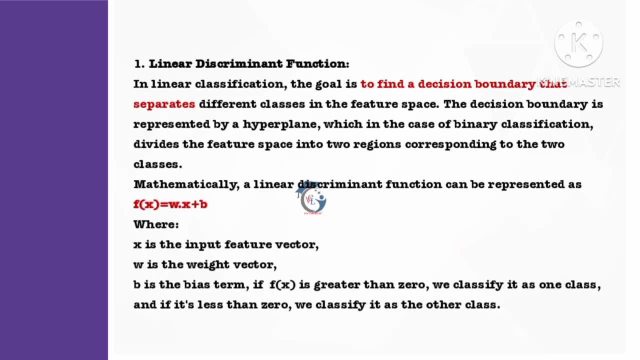 ok, so again, the best separation or decision boundary- we can say this somehow- linear discriminant functions. so I have told you what we will do after discriminant function. we will find out the decision boundaries now. we will do it with some features when we put that line. 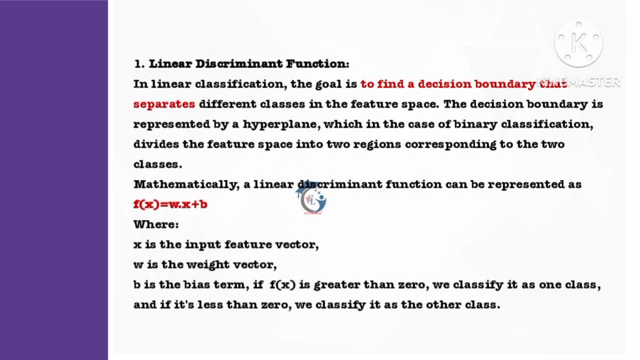 if that line is linear, it is linear discriminant function. ok, so when it comes to linear, we will definitely use this formula: y equal to mx plus b. you can also say that y is f of x in some function: x, we will do some function and we will generate y. 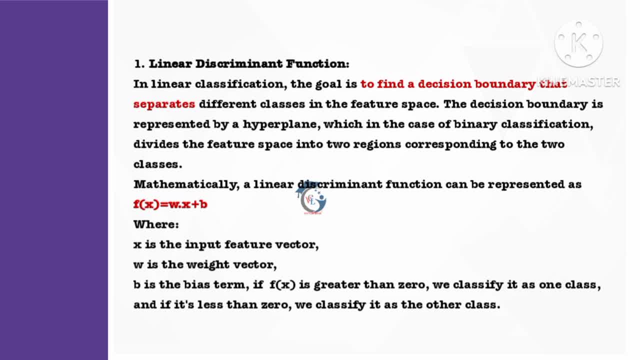 y or f of x, mx or wx, any variable you want, you can put it. ok, what variable we will put according to that, we have to give the explanation here. so x is the input features of the vector input itself. 1 or more than 1 may be there. 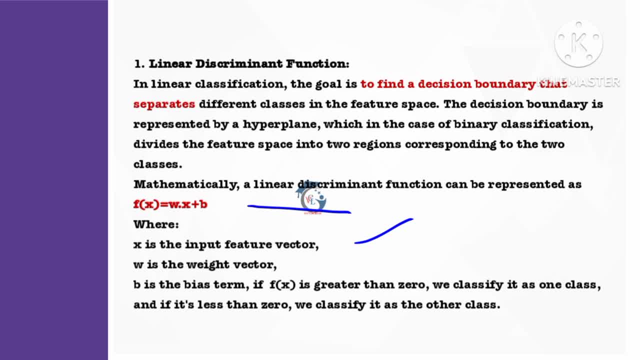 in that one input may be there many features and w is weight. what is the weight of that input? b is bias. we have already studied what is bias: y, y or f of x. we have to find out this: that value from 0, how it is less than 0. 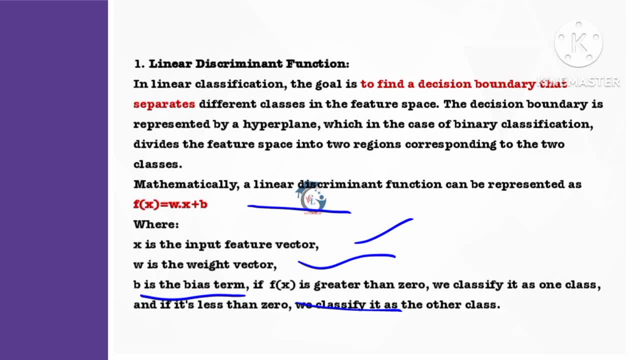 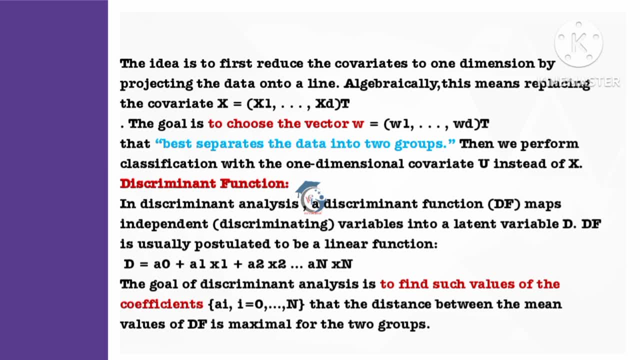 that is one class equal to 0. that is one class. we can classify it based on values, based on discrete values. we can classify it. ok, now I will explain how to do this. ok, as I told you, this input vector is more than w1- 2. 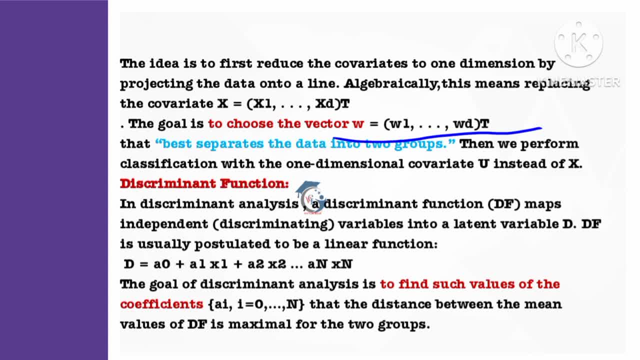 wn. if so, our best separation can be done in two groups, like many groups. ok, so discriminant function. in short, we call it df. so df is d equal to, as I told, 0, a, 1 X, 1 in the mother. okay, more than one. variables are mother. I'm in the 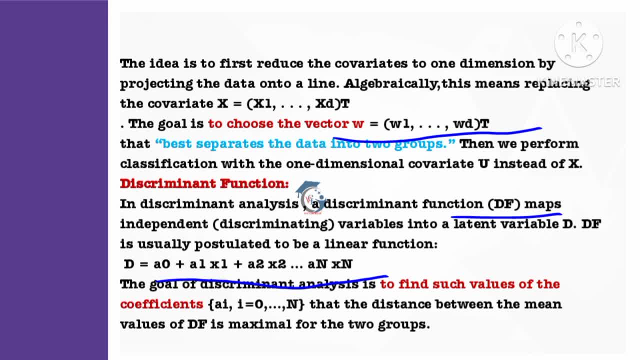 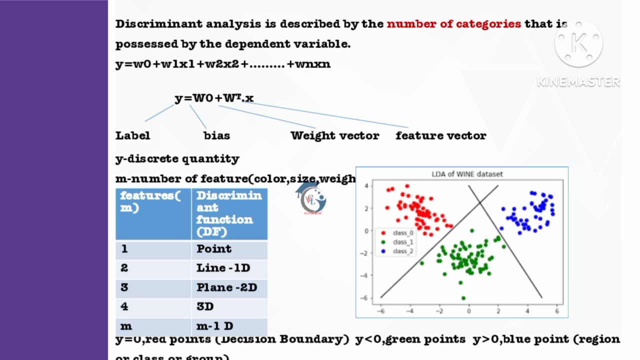 mother come. so the goal discriminant analysis, or the main goal, when they in the values, coefficients of, find out Pantana in the coefficients, find out panning other mean values, find out panning amount. in the DF, distinctive functions on the to find out. panic long okay, discriminant analysis lab, it's. 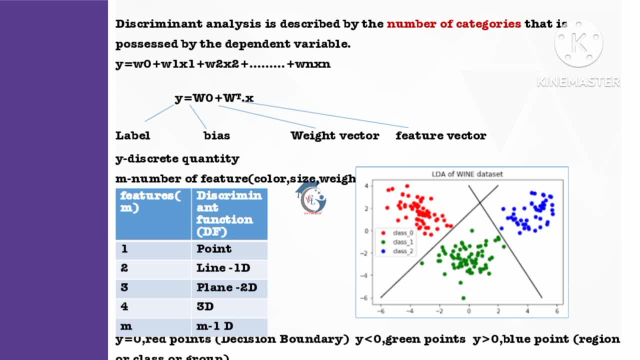 described by the number of categories, every number of categories, when the class by Pantana being a, nor example of seven, but not being a y equal to in a formula, it goes so more than one variable in the repair, it a pre in the variables in the shot, or so, Donna y equal to w 0 plus w, transform of X in. 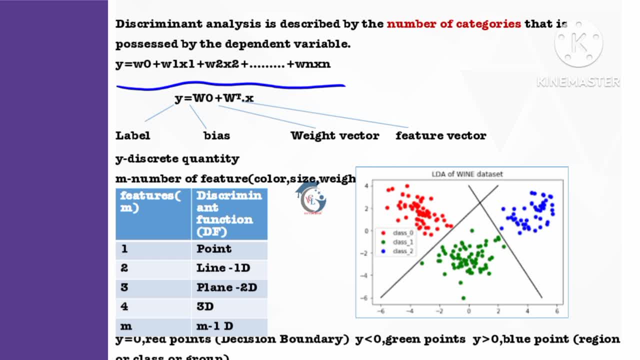 Kuroko. okay, so you will have y of being or the label. next, w, 0, mother- it's a bias- and weight vector, w- transpose and X- another feature vector or input variables. okay, um, um, y, equal to the discrete quantity in the mother of the find out Pantano. 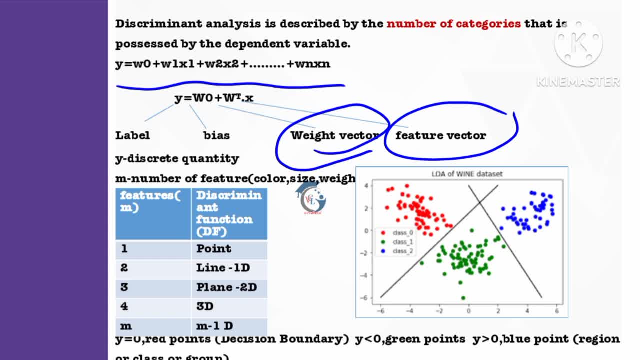 you know. number of categories, so younger the number of features, so color. which in my name, a puffer example in the, put in your mind. I read the line here from now: green color, blue color, the color in the balls over, maybe I didn't feel panana color, which one long size, which upon line, or a way to judge it. so you 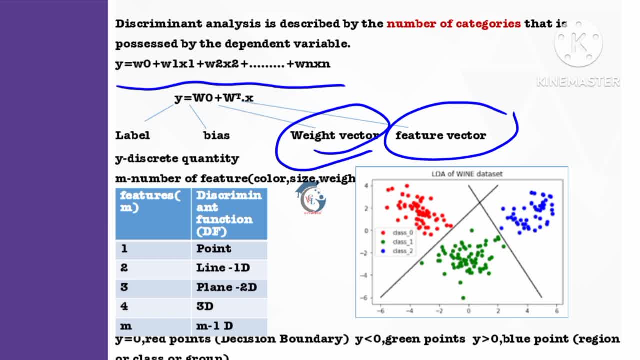 have a number of features. now you spend rain, that is yum, okay. so if a number in the features will see discriminant functions, say if deep and long? well, features, one, a one and a color amount, which I didn't feel and I have been over points for them. but color, you know, size, even chip and 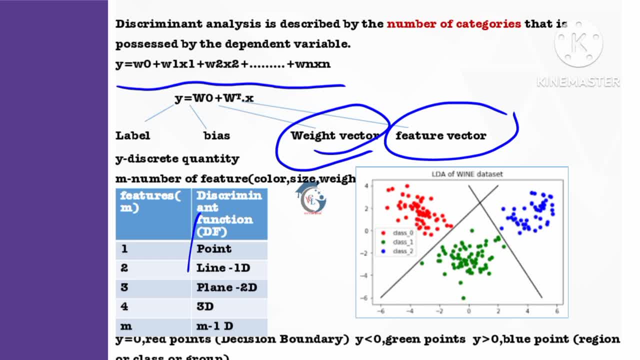 ramming it up a to other features to, that is yum. upper D of discriminant function on the single line, I do come, okay, I mean single dimension, or line which panel. so it features three recovery. now, two-dimensional features for my three dimension. likewise, how many number of features we are using, that is yum, yum. 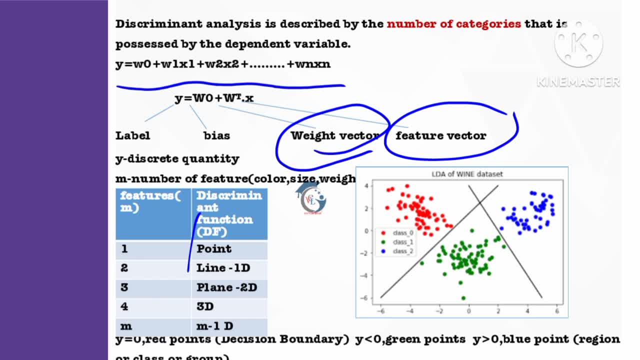 minus one dimensional 11, the mother we pond wrong. so in your boy, equal to 0, hyperbaric and the red points. and I calling now either and the order, this: either work class green, lower class, it will, our class it every panel on a way called zero, Mark, like color, and they be. 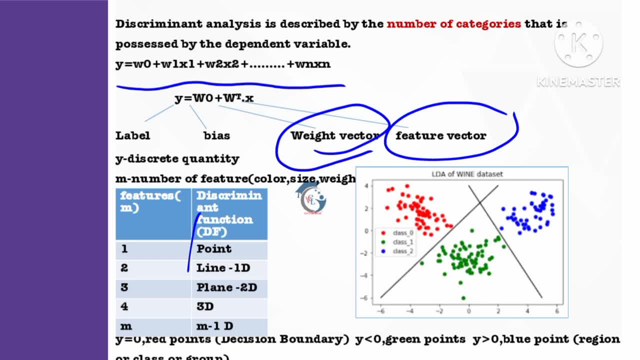 the bent in a little in the code colors in the married fly the lower boundaries, boundary or it's a region and the space. cool on the weather I'm gonna next we had at the classroom, are they didn't? our class 0, 1, 2 in the Maiden and good. 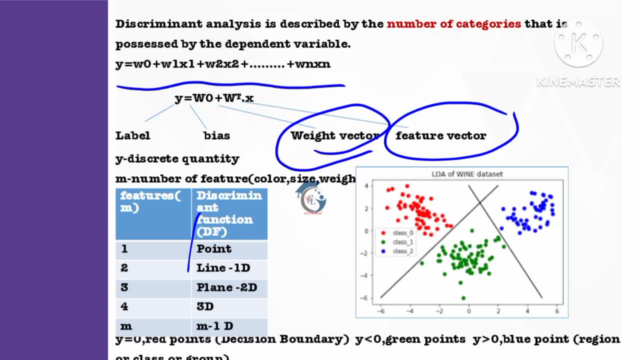 clock. okay, in the first name, input, data set, a input, a good good. on the data set layer, learn number of data class. we can beautiful親an is because we can be the some conditional based on mother, on the class by pond. wrong data will feed paneer to code paneer are the graphical, a visualized data which lies panel. 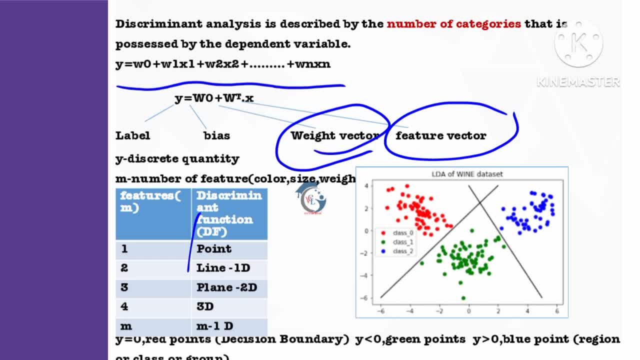 copper and I will open up. okay so DV leather mother, but it should go every day to explore Pano, a place where I spawn on the visualization, like graph mother generate of whom, or in the Murray points, generate a home based on that trauma, on the, in the analysis, in the learning model on the day, improve under 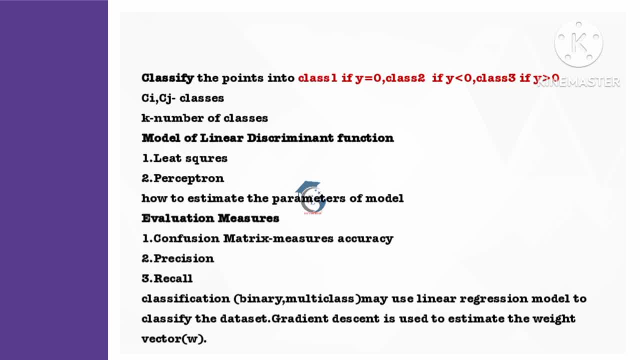 so if a based on y values, if y equal to 0, up in other class, y less than 0 or class gradients in or class in the madam panic like a mother. it's a number of class on a finger number. three categories is funny, for likewise so. 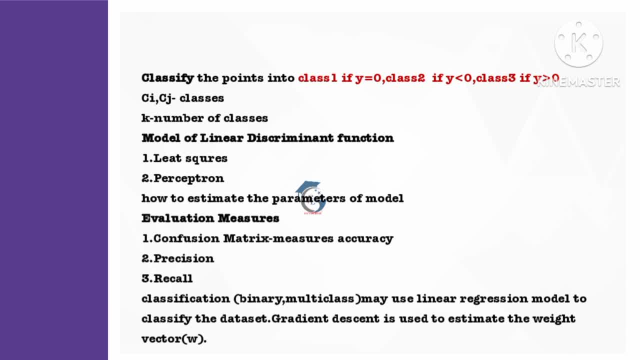 model of linear discriminative functions, analyze panel is square and perceptron is pond wrong. and evaluation measures every the model, every better either, copying every measure, panana, based on confusion, matrix and precision and recall, these are the methods to evaluate the measures of the models. so classifications to means binary and more than means multiclass, and for that we. 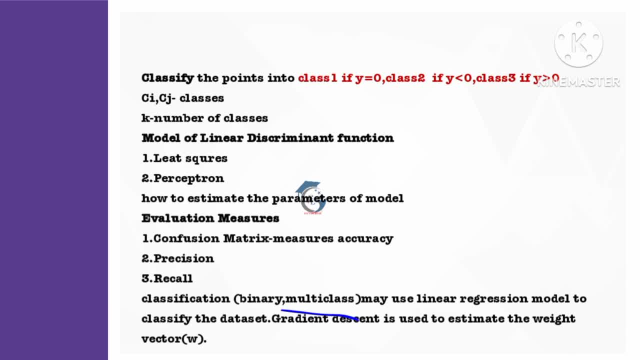 can use a linear regression models for classifications for contents of class we pondered to. we can use the linear regression models to classify the data sets. okay, based on it's based on the weight of the input variable, so the way it is represented as a W, okay either way. number: path of the Lamina. 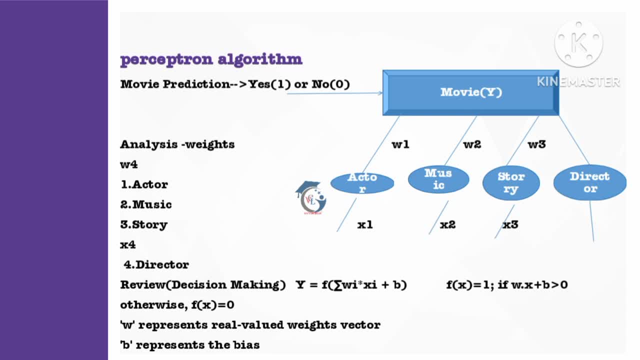 discriminant function, so this can function in a people or other path, of course. so the next topic is perceptron algorithm. suppose the trend algorithm is also for decision-making? it's mostly used for binary classifier. so binary classain means that is the to classifications won't be yes or no, true or false, likewise okay. for example, 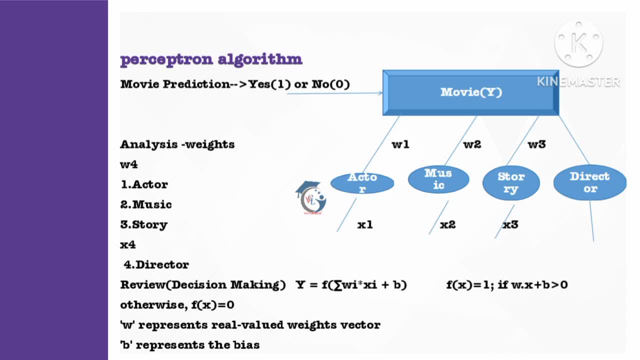 old, a more weak polar Politics interested Konami, which coma other than their own options. so we, even our car, would put a number come yes or no for marijuana bringer. if you have a device, a panorama, and be impacting now based on this, and I based on this, if an input in another turkey, I've been putting the actor in. 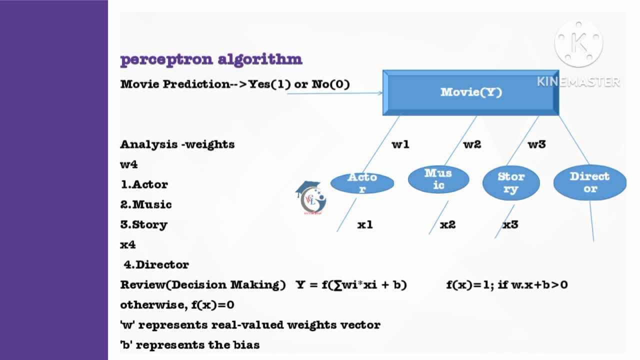 that turn on of the film copo and in order for a tractor in a pomata of the intermarital, a decision in a poem. sometimes music better. I'd go park lombina illusory. I don't break other music. a pericel about story. control my. 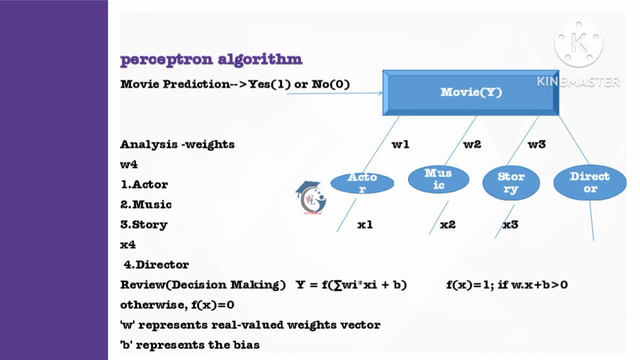 thrilling, I'd go up in a poker on. and, director, you were super. I'd para ever have any part of it on the Maori. so you know, basis lemma, decision, a decorum opening or other, that is, input features x1, x2 and x3. okay, so more than features. 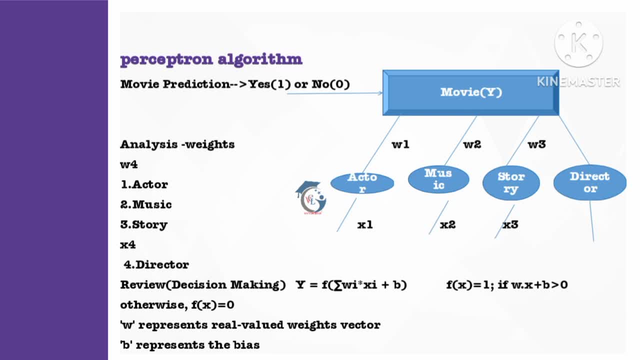 based on a decision made from, and the weight w1, w2 in the money. for what's weights I mean? uh, if a worry or a category, much in a decision, it come down. actor and I put a tractor on a film for a mean, and now number two. 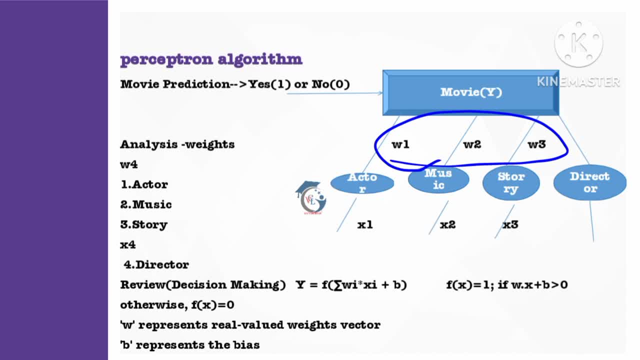 purchase actors or a film sale over when the flap. I'm a part of a toshirika Maria, so weight age of the- a lot of the features from a weightage portal. I thought I mean value to the decision. it can be polama when I'm a be in it so active. core weight age. 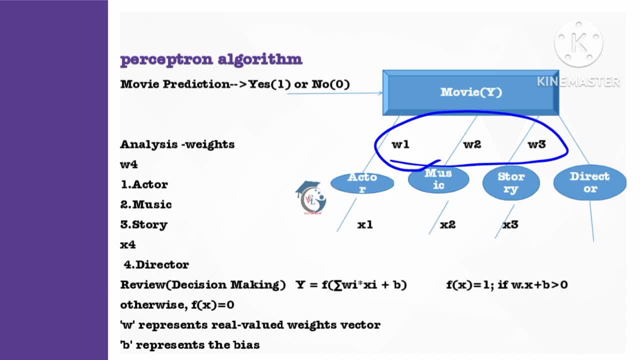 music or weight age story. core weight age director for weight age in values, and I'll put a zone, a mean value editor and the mean value number load, a threshold value of it. a man, okay, why you the cup in a number decisions, yes, near upon or no, near upon King law. I even touch it through Amma be now. 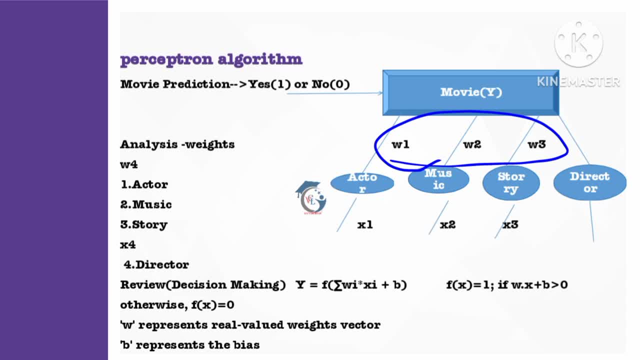 condi part review pop. oh, okay, then I'm load assumptions, lemora, decision it through on and other sort of opinions review. but the other land, or either condo room. so if a theory, the x1, x2, nine happening or the w1, w2, that it's the weight age. so either, to summarize to the 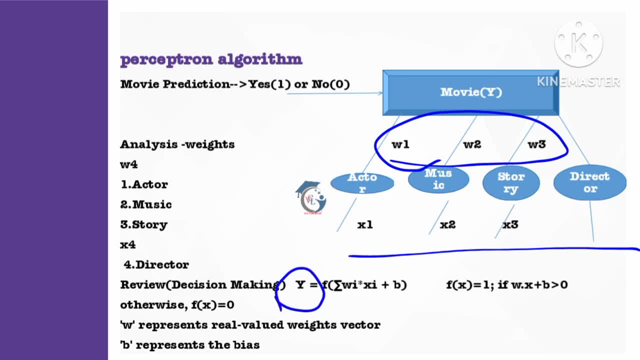 way weighing. that. it's a decision. so you have data corona F of other function apply pond wrong. so WI star X, I in the render to a weight age, you and the variable you multiply penny plus bias, one that you know, Matt Pano, no matter, could have them wait. okay, so if the F of X or the Y value is 1, 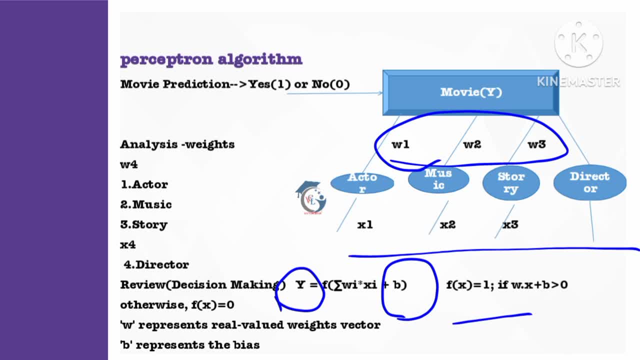 Abhinav. yes, Nampola, be not, though, if the value is greater than 0. so, on the weightage values, number, find out panel. okay, it every find out panel are being, rather than I'm on the mean square method, least square method, slalom of. 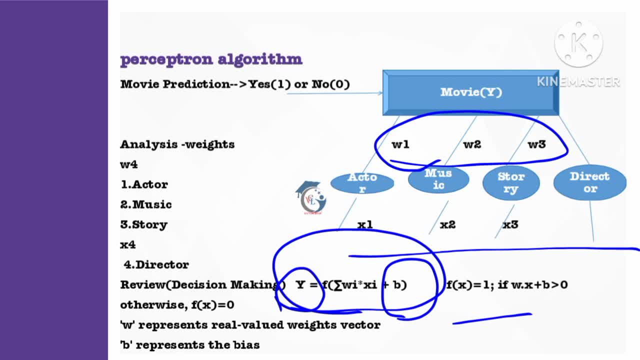 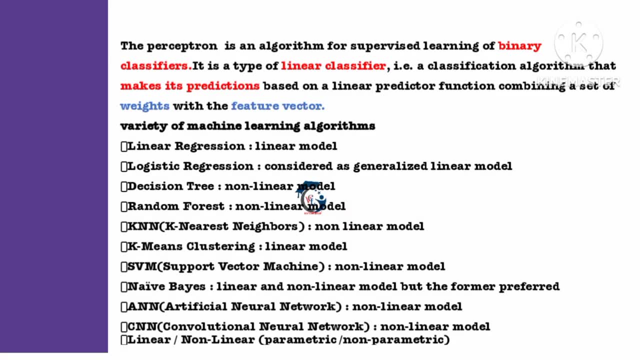 fine, but it's your phone, okay. so W a bring other. it's a weight age, be a bring other bias. are you clear, okay? so the perceptron algorithm is for supervised learning, mainly for binary classification, so two options were more than I used. easy, and the method is funny. I'm a panic a medium, so it makes the 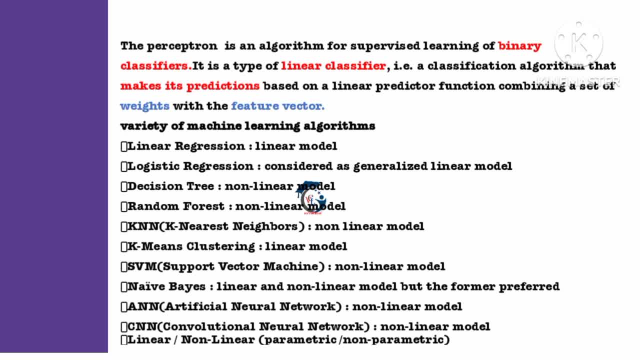 predictions. so based on the weight, age and input features. okay, so many variety of machine learning algorithms are available, like linear model, regression model, decision tree, random for us, and KN and K means algorithms. some of these algorithms or comes under the linear model, some of these are nonlinear model. already we discussed what is linear and what is. 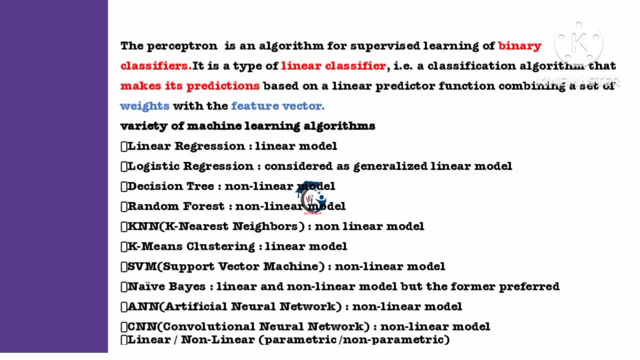 nonlinear models. so based on the inputs and features of the inputs, we can decide which algorithm I'm. a use panel are based on which algorithm or the decisions on the accurate I'd come better. I'd comprehend other than you know decide panic law. okay, so next are the characteristics of perceptron. so either parting now, it's a. 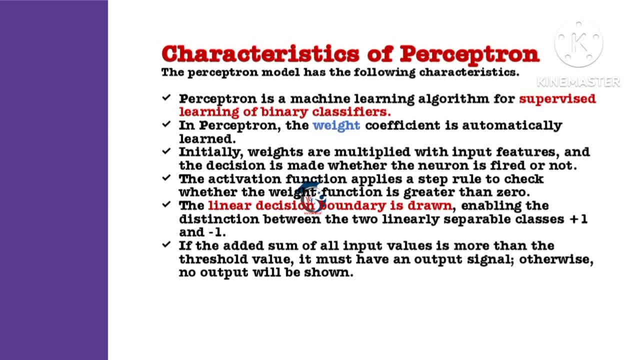 machine learning algorithm. it's a supervised, mainly used for binary classifiers, and weights is pond wrong. okay, so we initially the weights. a beautiful other weights are on the turn input features or a multiply panel. more answers on the world other than number of decision boundary on the to find out. 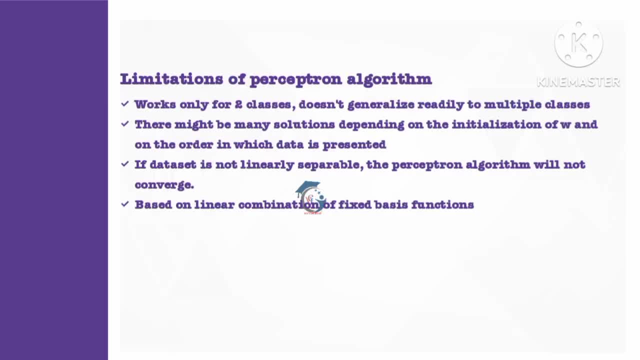 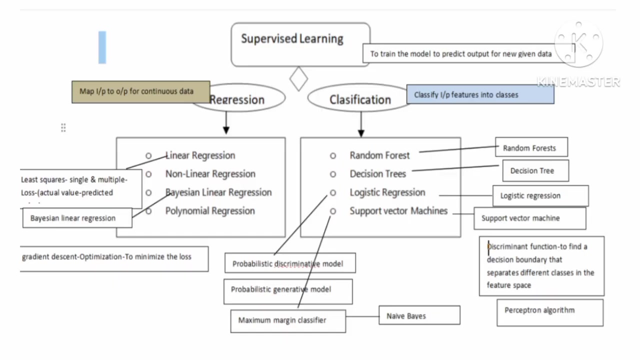 pond room. so these are characteristics and limitations of perceptron girl. it's only work for two classes because it's a binary classifications okay, and so this algorithm is useful for linear classifications in the next classes apart long. so next, in the diagrams kunjipatakou, my down the actual. 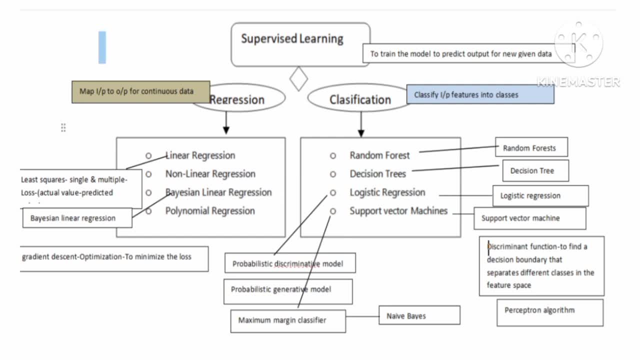 summarized, so supervised learning. other model: a train panel output of predict, ponder the koho for some new data. so there is two methods: regression, classification. regression is mapping input output variable, it's work for continuous data, and classifications for linear classifications. it is useful for numerical data. okay, and it's class be upon when the category global being. 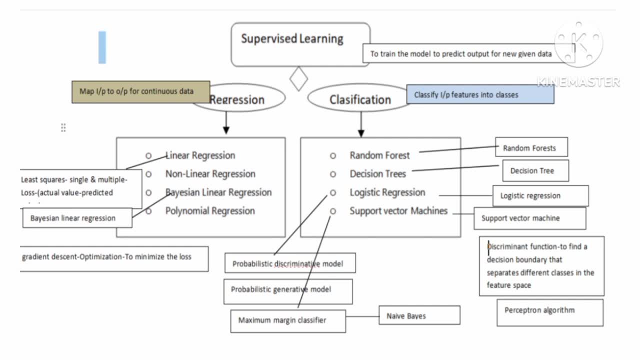 ordered. so regressions, cool about in a linear regression, nonlinear regression base. in America, linear regression methods in the least square methods use for no. so single and multiple variables is funny, sorry. and base and linear regressions on the formula is funny, no matter, find out for no. then gradient is. 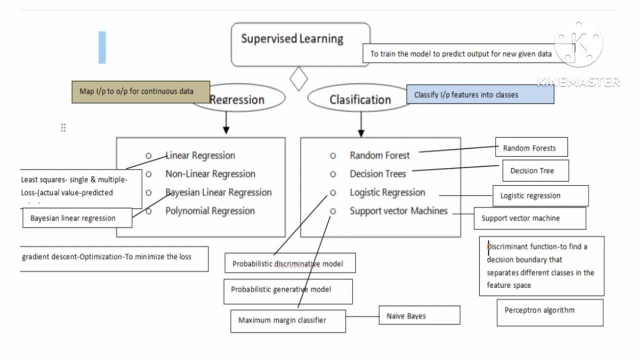 this and is the optimization algorithm is to minimize the loss. may miss. funny. other predictions are better. a condo at the column of under the next classifications: la patina, maca, decision, tree, logistic, a dilemma in minimum detail, a proper room. so from a part of the discriminant function and perceptor. 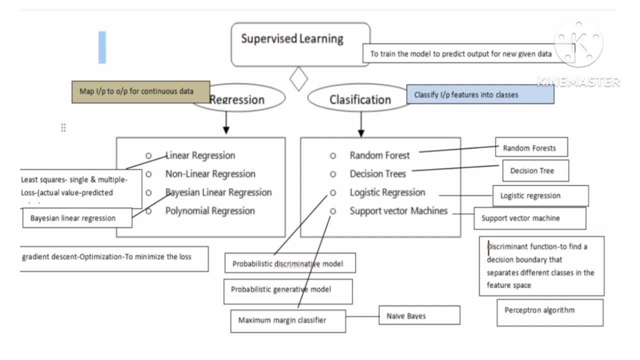 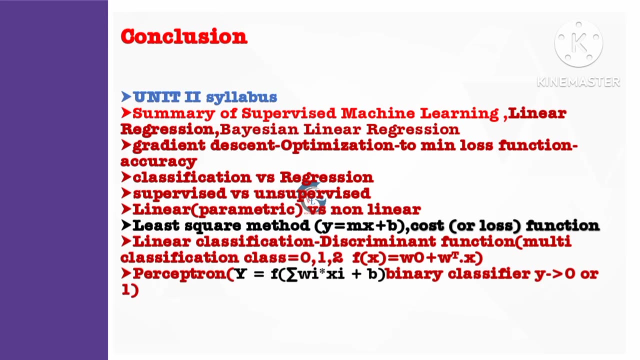 algorithm discriminant functions to find a decision boundary, a linear and schnell in a different partner. okay so in a question, the basic remaining regular addition to logistic regressions are the even, and I'm an extra to talk about our topics. okay so the conclusions. second unit orders- levels, part of 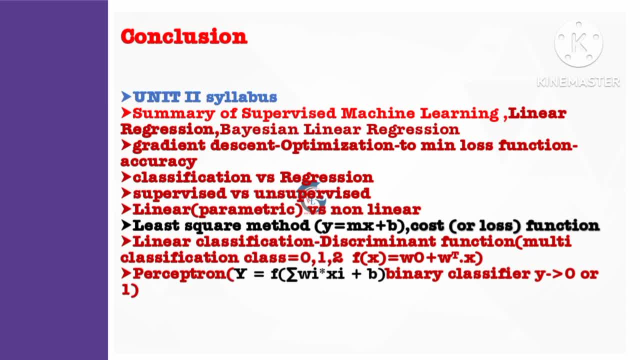 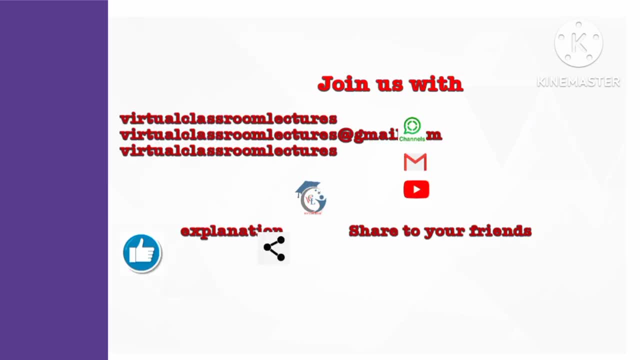 common summary part of our previous topic: order and classification, regression, supervised, unsupervised, linear, nonlinear, early square methods. you know, my partner on discriminant function and perceptron is the new topics. okay, now please join us with virtual classroom lectures. you can join with a whatsapp channel and gmail. you can ask them doubt or you can use gmail. 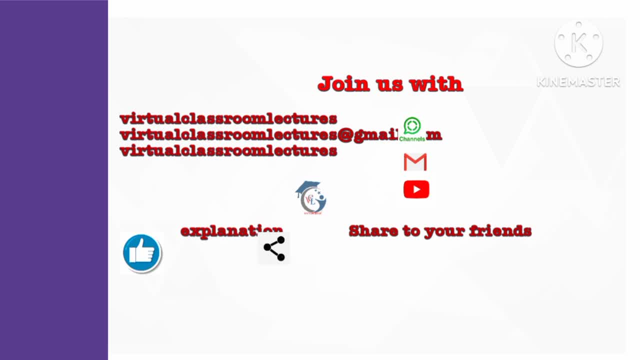 ID and if you have any comments, please post it in our comment sessions. if you like, please share this content to your friends. it will helps to get good marks for your friends. okay, thank you.